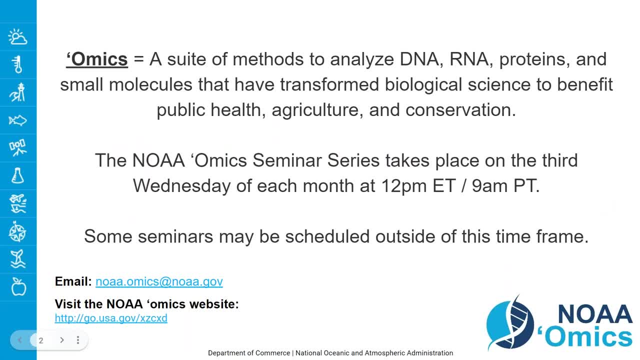 OMICS, which is a suite of tools used to analyze DNA, RNA proteins and metabolites, has become a large priority here at NOAA in the last several years. We established this seminar series in an effort to increase transparency and collaboration and highlight the incredible 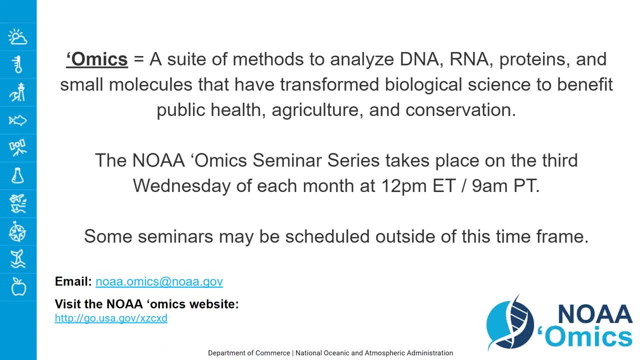 OMICS-related resources. Thank you, Thank you. Thank you so much for taking the time today to do such interesting research anddaless foundation for global marine research currently underway both within and outside of NOAA. The seminar from this series are made available on Youtube and posted up on our OMICS website. 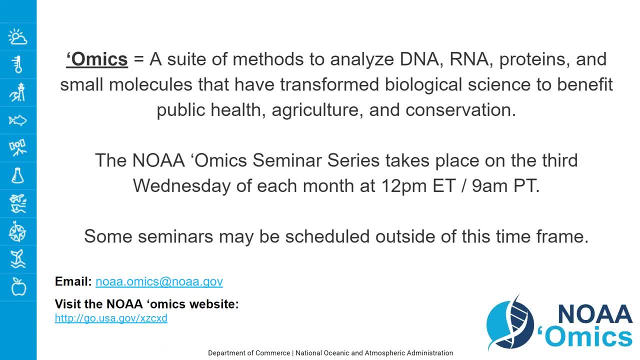 There is a link to the website in the chat now for folks who want to go and view past webinars. As participants, you are muted, but feel free to type questions into the questions for staff box throughout the presentation. At the end I'll read the questions for our presenter. 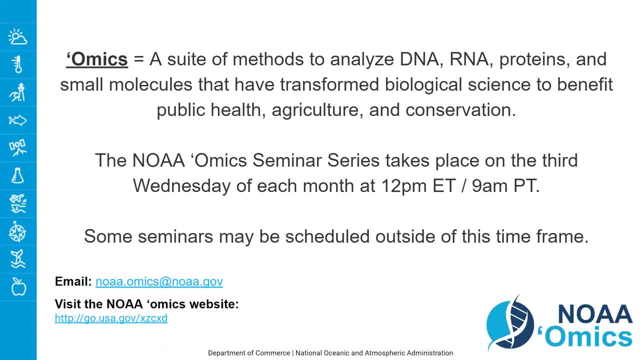 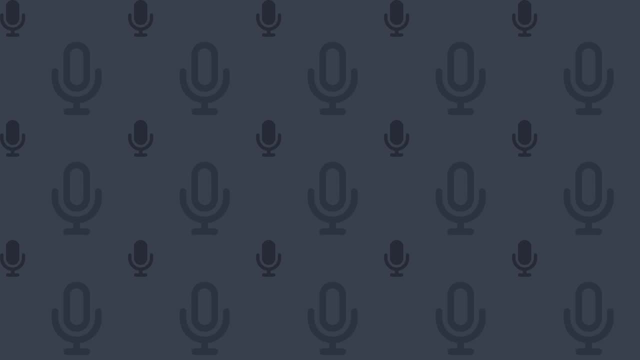 to answer: biodiversity monitoring, your partnership and innovation, presented by dr Luke Thompson. so, Luke, I'm gonna go ahead and give you screen sharing permissions and while you're getting your presentation set up, I will introduce you to our audience. okay, so dr Thompson is an associate research professor at the 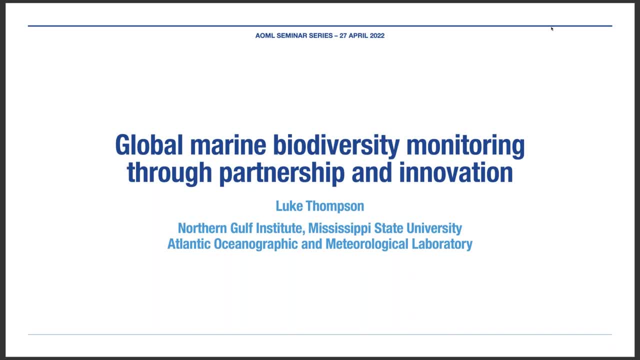 Northern Gulf Institute at Mississippi State University and NOAA's Atlantic Oceanographic and meteorological laboratory, or AOML, in Miami. Luke received his bachelor's degree from Stanford University and his PhD from MIT, both in biology. his current research focuses on marine systems, from microbes to fish to mammals, using omics methods, especially DNA sequencing. his lab is 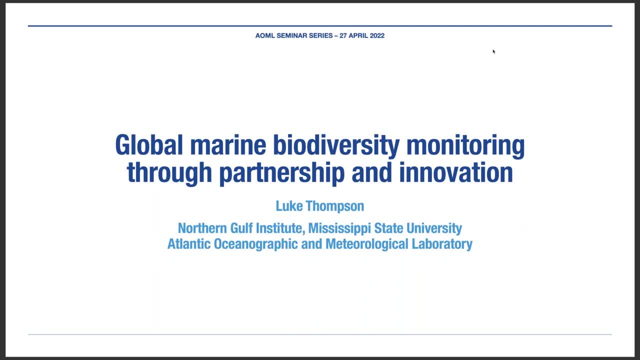 developing methods to facilitate high throughput environmental DNA sample processing and data analysis and applying them to monitoring and conservation efforts in the Atlantic Ocean, Gulf of Aegean and the Atlantic Ocean of Mexico and the Great Lakes. so, Luke, thank you so much for presenting today. I 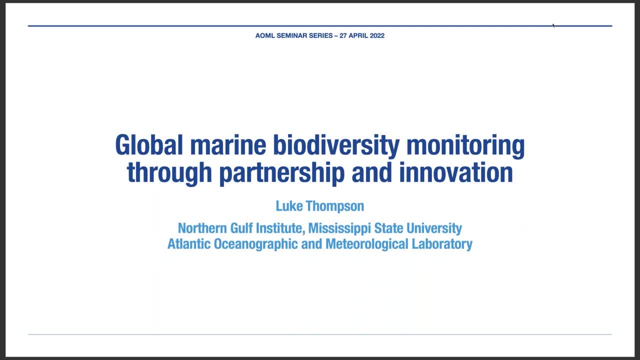 will now pass it off to you and we can see your slides as well. great, Thank You, Katherine. thanks for the invitation and the kind introduction. so, yeah, today I want to talk about some of our work at AOML and, in particular, focused on global marine biodiversity monitoring and the partnerships and innovations that make 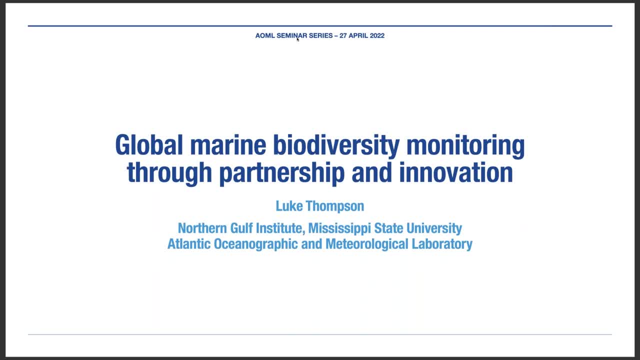 that happen. please disregard the little header there at the top. I neglected to update that. so today is July 20th, if you're keeping track at home. and yeah, as Katherine said, I'm at NGI, which is a NOAA Cooperative Institute through Mississippi State University, and I'm based at the Atlanta Oceanographic and 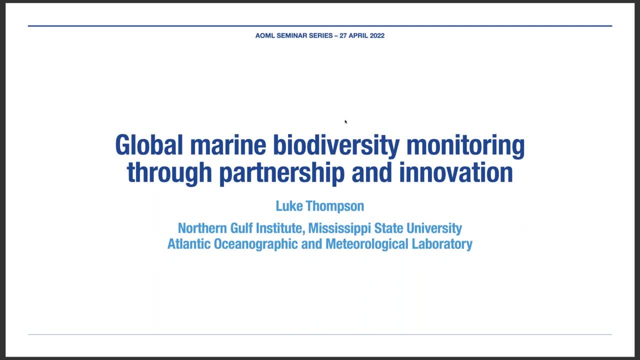 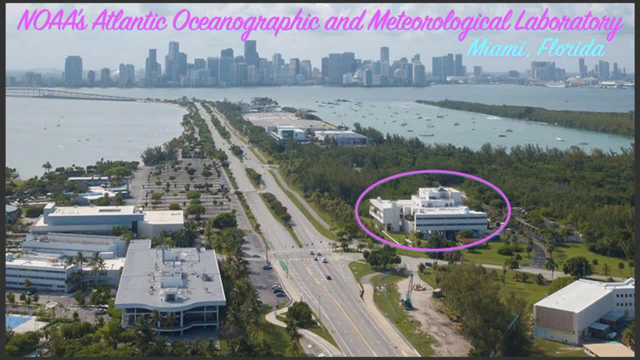 Meteorological Laboratory in Miami. so to orient you a little bit, this is what our lab looks like. it's. it's on Virginia Key, off the coast of downtown Miami. it's this white building there, circled in pink, and it's a great location. we're right on the Atlantic. 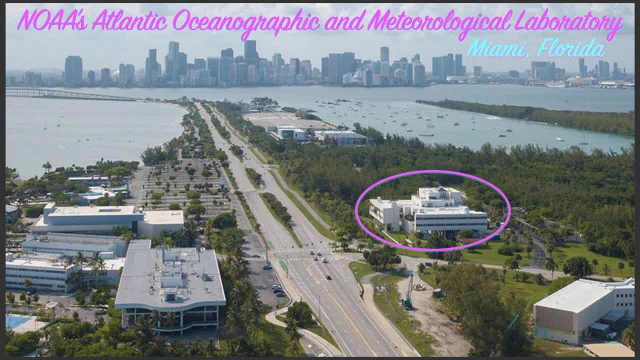 Ocean in Biscayne Bay. we're located across the street from the University of Miami, which has a lot of additional resources for marine science, and, yeah, it's a great place to work. in fact, we're actually in the process of hiring a couple new post-docs, and a technician and a project manager. 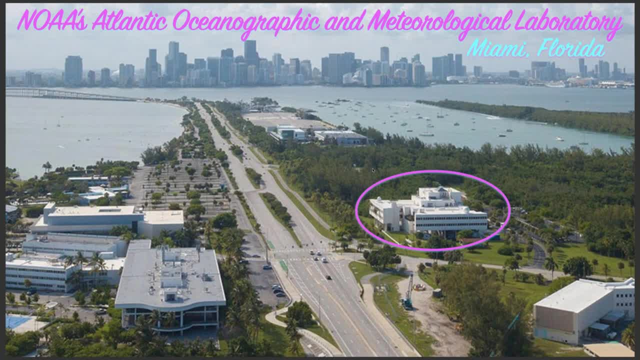 if we can get that all through the system. so if you're interested in the work i'm talking about and you want to get involved, please let me know, and we have some additional projects related to carbon export and ocean acidification that i i won't really even touch on today. so there's a lot going on. 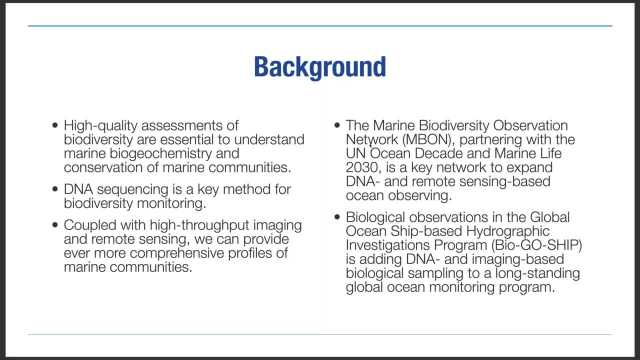 so, as a background to to my talk, i wanted to just lay out a few things. i'll go through this visually in the next few minutes. so, um, the main thing- uh, sort of in in terms of background- is that we need high quality assessments of biodiversity to understand marine. 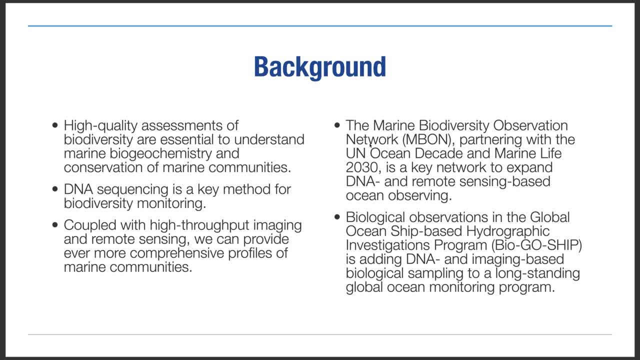 biogeochemistry and and to conserve communities. we need to know what's there to be able to, obviously, to understand it and to to protect it and conserve it and be able to measure it over time, and so dna sequencing has emerged as a key tool for for monitoring biodiversity. 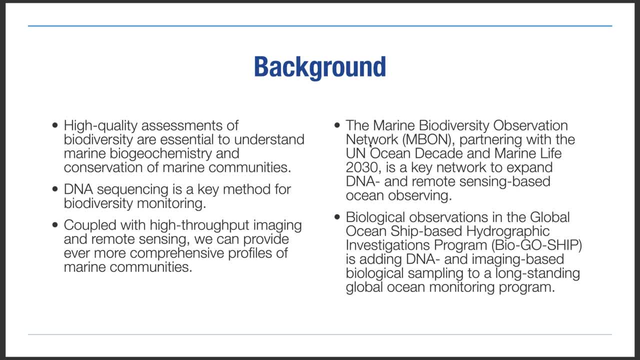 and it's also being coupled with high throughput imaging and remote sensing and that way we can get a really comprehensive profile of marine communities, and there are some efforts underway, uh, to do this. but there's a lot of room for improvement and expansion. so a couple of the um, the networks that we're involved with that i'll talk about today, are mbon, which is the 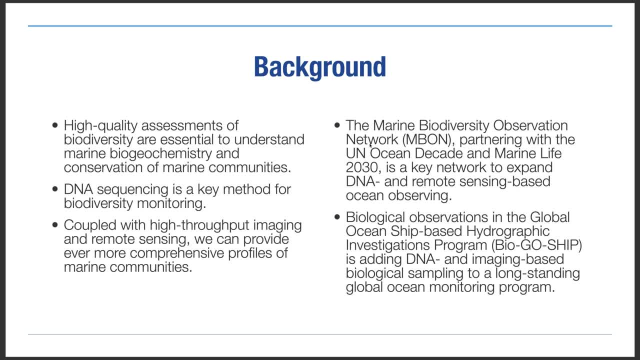 marine biodiversity observation network and that's partnering with the un ocean decade and marine life science organization um, in a way that is, you know, connected to more of the Państwo sea, notre hybrid research institute um, which is, uh the uh, the main project um, and that's where we 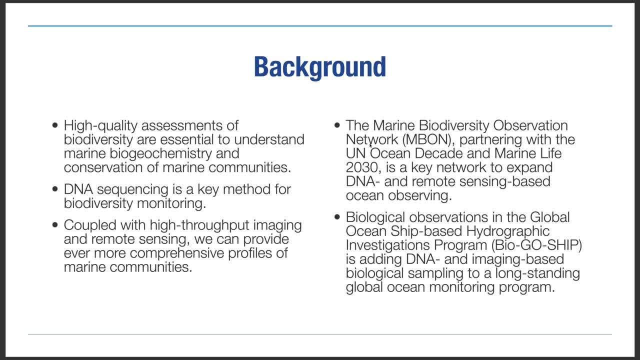 work with the marine biodiversity association, um for um, starting to understand um, the, the mineral history and the ocean, and then adding kind of my own tools that we've used since the beginning of 2013 and so that's covered. so based biological sampling to this long-standing global ocean monitoring program, and i'll talk. 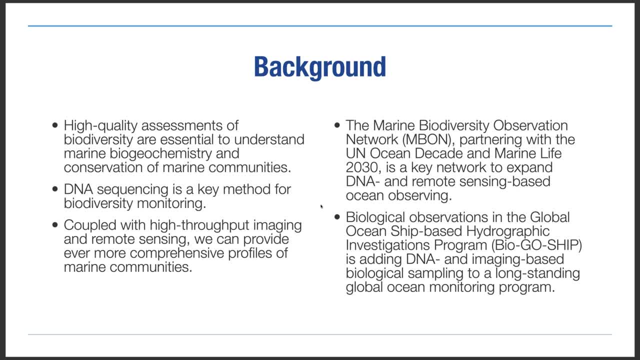 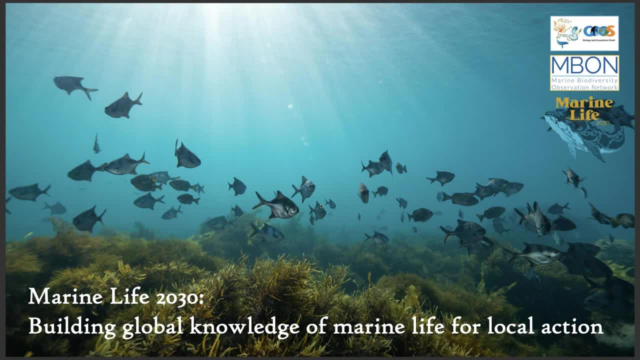 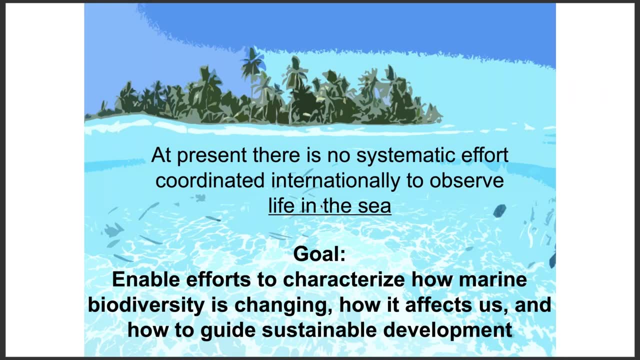 about both mbon and biogoship today. um so a little bit about marine life 2030, and i want to thank enrique montes at awml for providing some of these slides. so the the problem or the situation is that at present, there is no systematic effort. um, 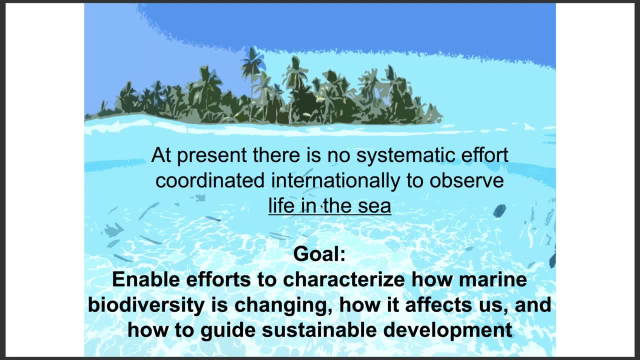 coordinated internationally to observe life in the sea, and so the goal of of this effort is, or the goal of of this, um, yeah, this effort is to enable, uh, efforts to characterize how marine biodiversity is changing, how it affects us and how to guide sustainable development. and so, as as a key example of this and where we're lacking, 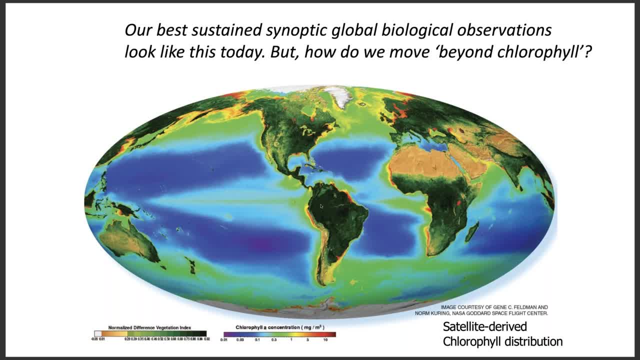 um, this is a beautiful picture of the earth and the ocean showing, uh, chlorophyll, um, or ocean color for the ocean, and vegetation for land, um, and so this shows you where there's the most primary productivity and and that sort of thing, and that's of course, really. 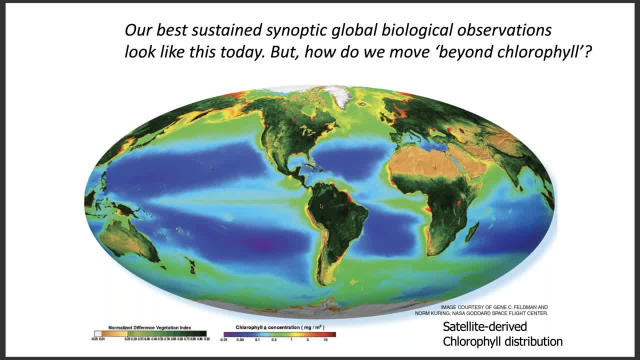 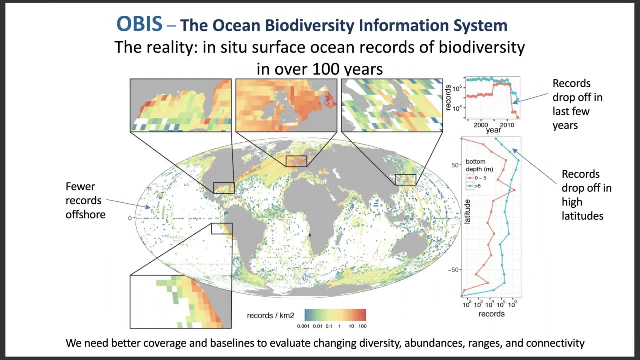 important information, but that's really the only inputs into a lot of our models for how we understand the ocean in in a larger context, when we integrate with fields outside of biology, and so this is, uh, definitely something that that we want to improve, and so, uh, for example, um, we do have some some biodiversity data that's stored. there's a very 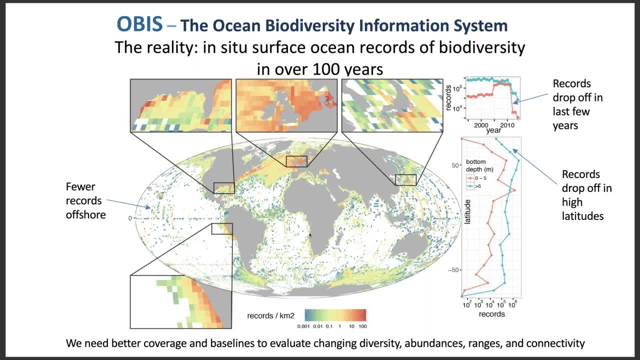 nice system called the ocean biodiversity information system, um, and it's containing um a lot of records about observations of um of different species and so forth in the ocean and um, but it's it's, you know, not complete as you can see in the map there's, there's some parts that 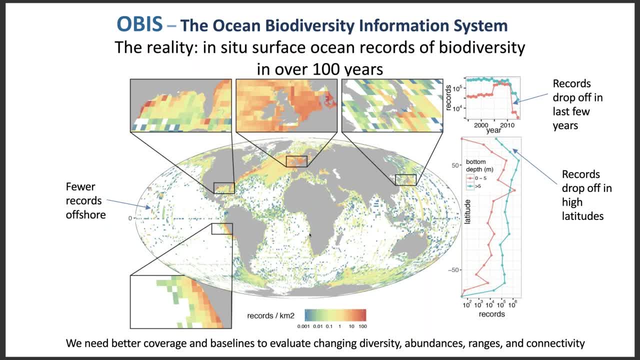 are that are pretty densely sampled. there are other parts of the ocean that are very, um, minimally or not sampled at all. um, there's been a drop off recently in um, in the number of records over time, as well as uh in uh, at certain latitudes there are fewer records. so, um, this is, this is certainly- 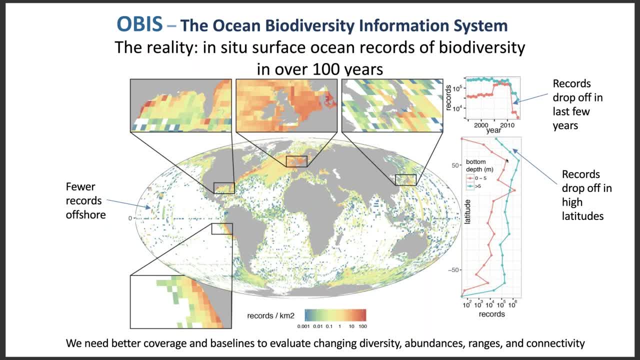 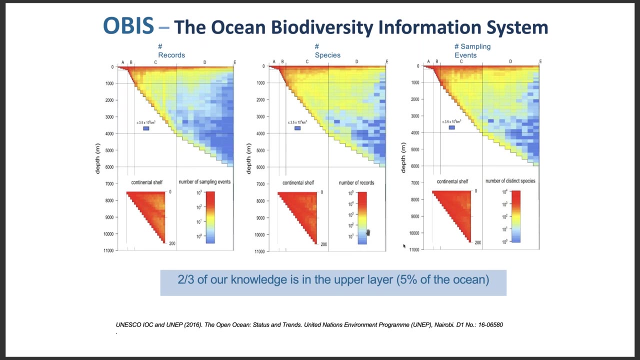 something where we want to improve coverage, um, and the baseline would that is: uh, that is the total coverage at a given time point. you know that to then track over time changes in diversity, abundance ranges and connectivity between communities, um, another example from obis is that as you get deeper in the water column, there's there's fewer observations. 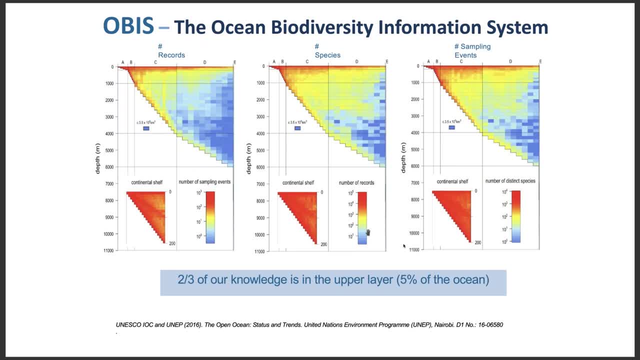 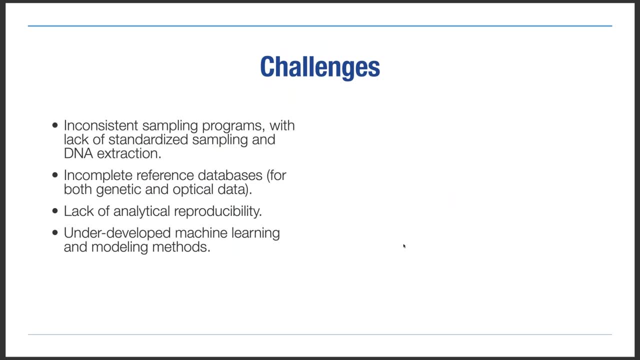 so most of the observations are confined to the surface. so, uh, to kind of go through the challenges in this um situation for uh, for global ocean biodiversity sampling: um, there's inconsistent sampling programs which i kind of showed you a little bit already. there's also um a lack. 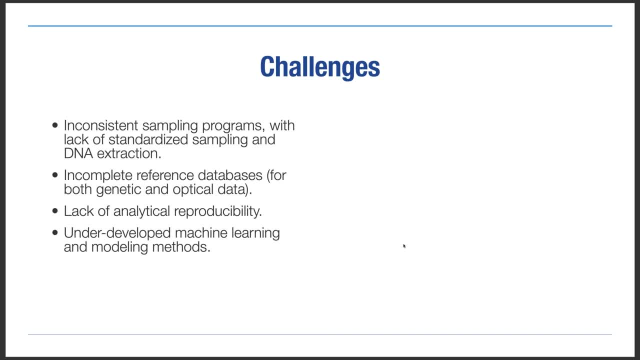 of standardized sampling and dna extraction methods, um. so when you're specifically talking about omex based methods or genomic based methods, um that's that comes into play. um also thinking about genomics specifically, um. so that's a little bit more elucidator for data extraction. we kind of 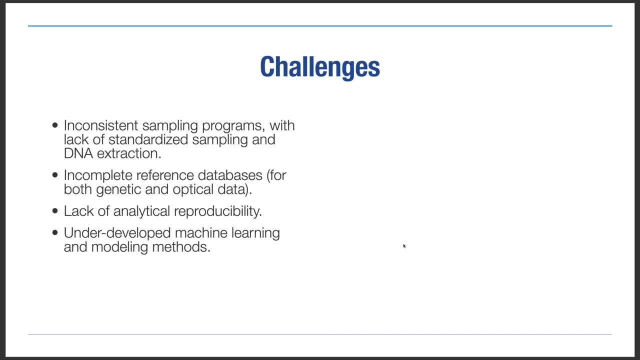 EQ was also trying to make this complex analysis um and also generate significant findings. but then there's incomplete reference databases, and this is true actually for both genetic and optical data, which i'll talk about a little bit in a little bit. there's also a lack of analytical reproducibility. 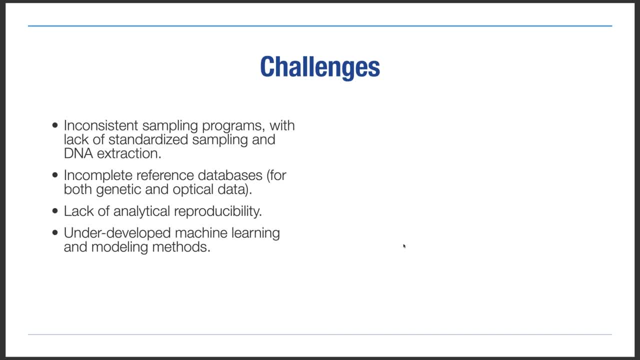 people using different methods, and also um, not even just reproducibility, necessarily, but also just um sensitivity and accuracy of of the methods that are analyzing the sequence data and the optical data. um, and then there's, um you know, sort of underdeveloped machine learning and modeling. 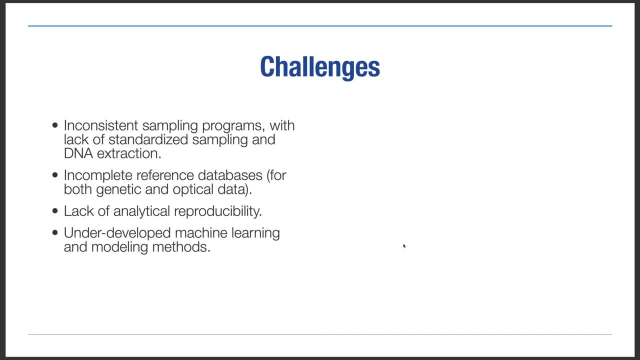 methods. there's a lot of capability now in in coming from other fields in natural language processing and image processing and basic research and machine learning and um and weather modeling. there's a lot of other areas where these methods are used more than they are in biodiversity and genomics and um, marine imaging and and kind of our, our neck. 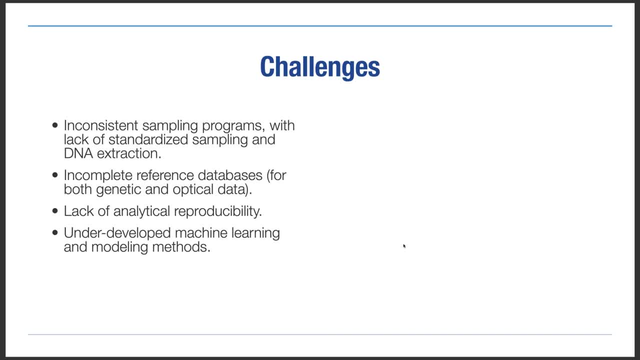 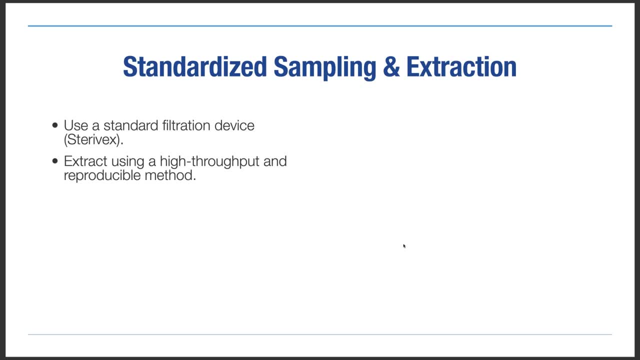 of the woods. so there's a lot of potential there that's that's untapped. so first i'll talk about standardized sampling and extraction methods that we've been developing, um developing in our lab. so these are some, some results from our lab that we'll talk about, and so 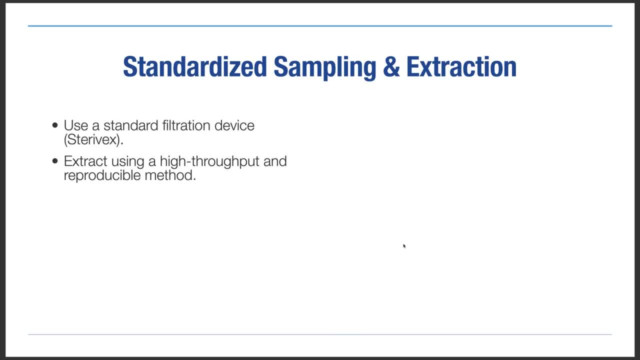 in this case, we? um the goal or the idea is to use a standard filtration method, um, and one that's emerged, uh, that's very commonly used, is called sterivex. uh, i i wouldn't necessarily say that we should use this for all um ocean sampling, because there's, there are reasons to use other. 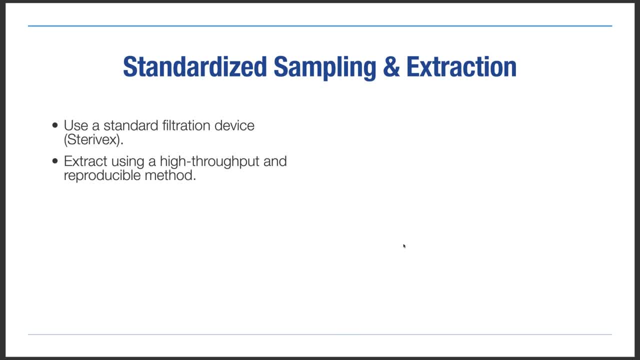 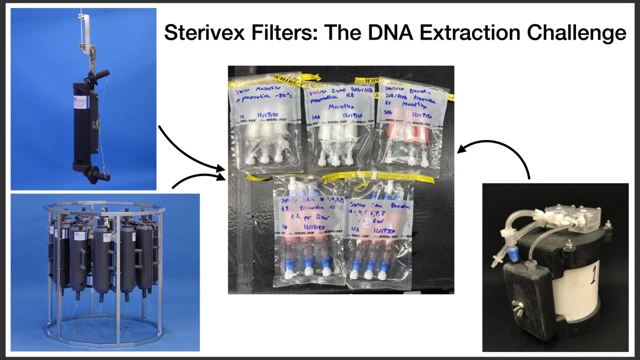 types of filters, but this is one that's emerged as a popular option and so that's the one we're using here. um, and we want to have a high throughput and reproducible um method. so the sterifex are these little filter cartridges shown in the center. um, these are um, these can be, you can filter water through them, and i don't. 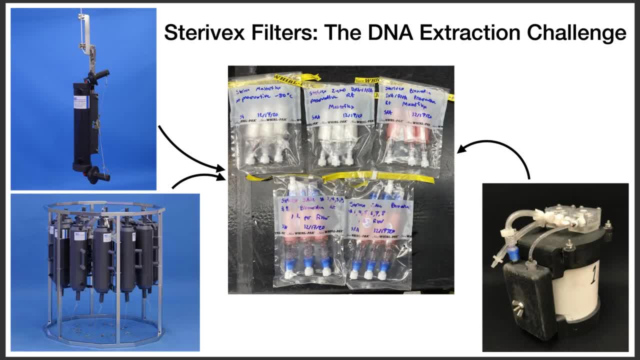 have a picture of the pump that we use, but we use a peristaltic pump to filter water from either a niskin bottle that's dropped on a line or on a ctd rosette that's shown on the left, or um collected via a, an automatic sampler like the, the sassy that's. 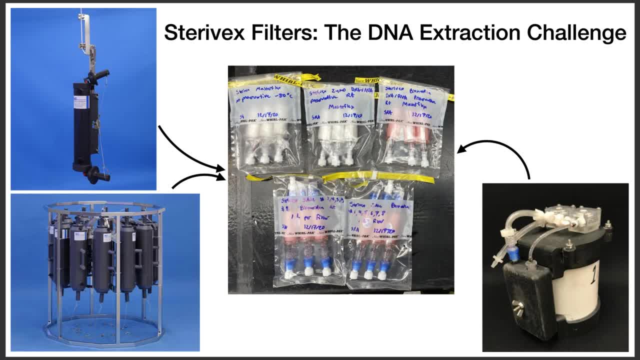 shown on the lower right- and i'll talk about that um a little bit later- and so, however you get the water, you then filter it through one of these sterifex filters and you maybe add preservative or maybe just run it dry, which is our preference, if we can. 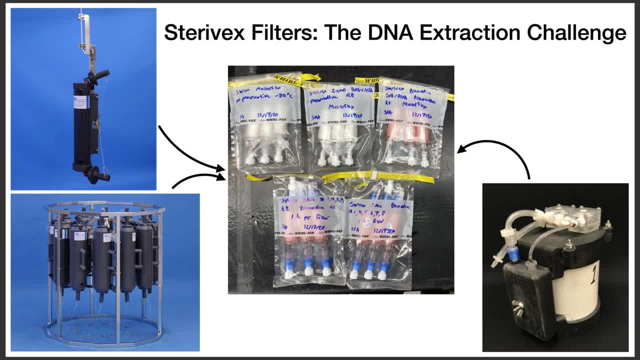 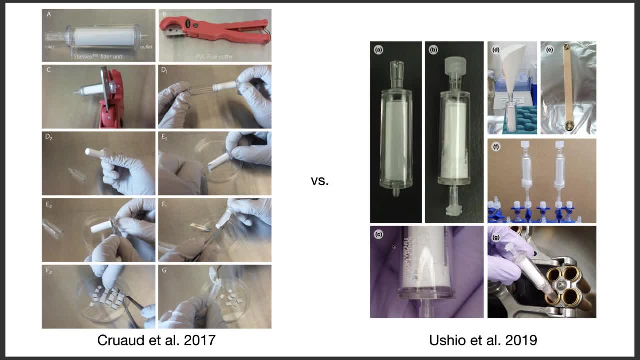 but now you have this problem of how to- uh, how to get the dna off of the filter. so, um, the traditional method was to cut those open and to peel off the filter and cut it into pieces and then stick it into an eppendorf tube. and it's very tedious, it's prone to contamination and it takes a long time. 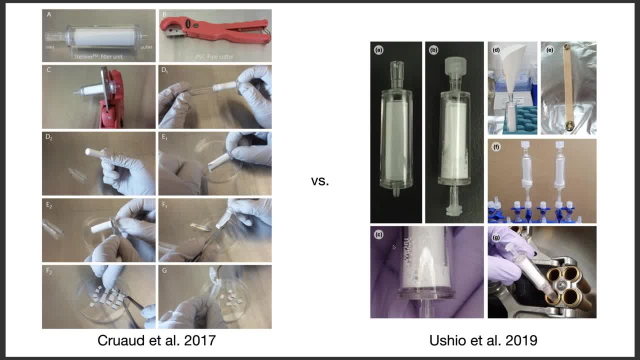 so there's been a newer method that was developed where you add, like glass beads, basically to uh, to the inside of the filter. you can do this either before or after you collect your sample. we do it after and then you do a vortexing, so a two-step, and you do the process of um. 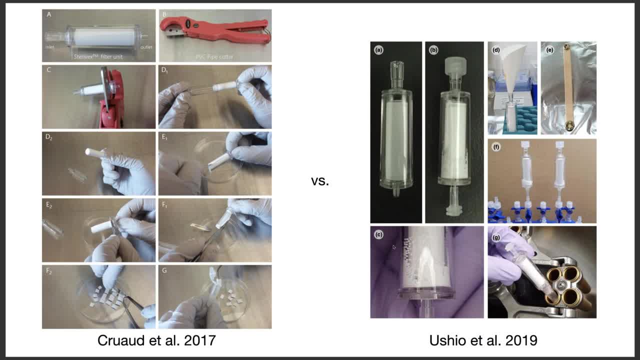 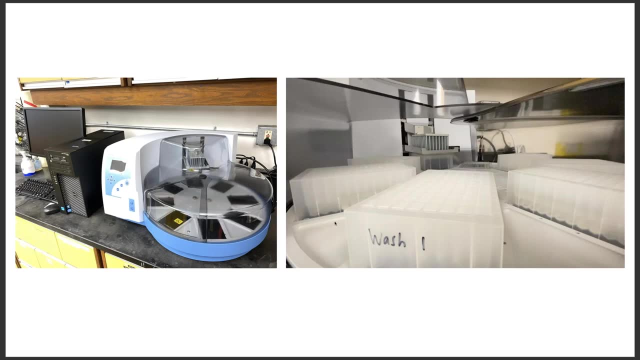 moving a little bit and then you do the process of, uh, kind of lifting it up, and then that will kind of chop up the cells and and give you a nice lysate. so so we found, so, um what we did in our group, and um this work was led by sean anderson, is to test this for some samples that were collected. 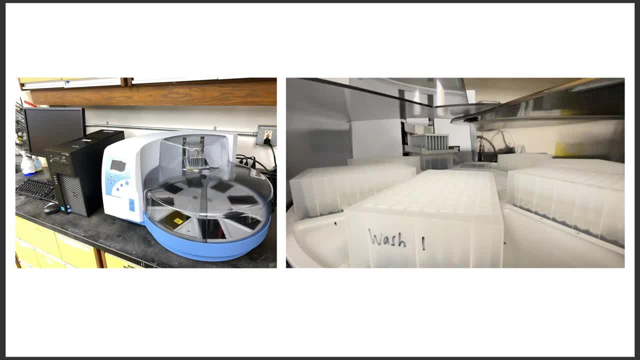 near um, near aoml. so we used two different um Kingfisher Flex robot without any plates on it, but this is a magnetic bead handling robot that we use to increase our throughput and on the right, you can see inside when there's, when it's loaded. with with samples it will. it uses magnetic beads that will bind to the DNA in the lysate from the sample and then wash, do a series of extraction and washing steps, and when you're what you're left with at the end is purified DNA attached to beads that you can then remove the magnetic. 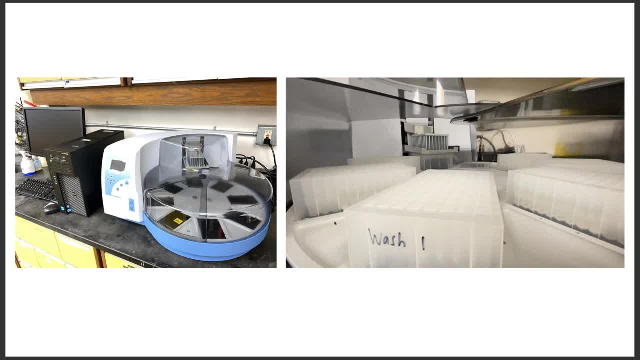 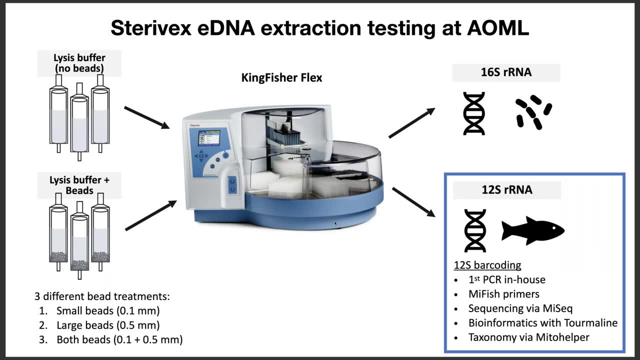 beads and just have your purified DNA. so it's a really nice, nice platform. and so what Sean did was he tested with or without beads or a different combination of beads? and then there was, and then we looked at the 16 s, our RNA gene of bacteria, and the 12 s are RNA gene of fish. so we'll show. 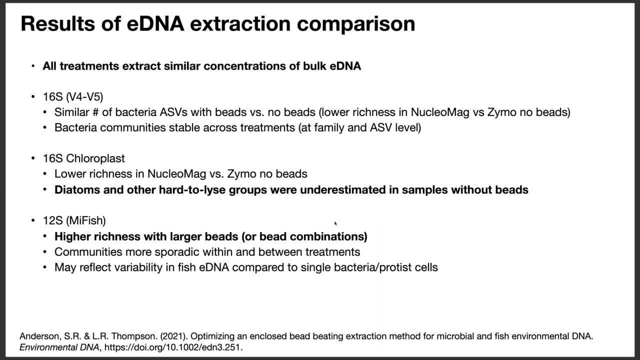 you the, the fish genes, today the fish results. the high-level results was that generally all treatments gave us similar concentrations of DNA, but the treatments were different, different, slightly different taxonomic composition and and we got better. we got better recovery of hard to lice organisms like diatoms with with beads, so using 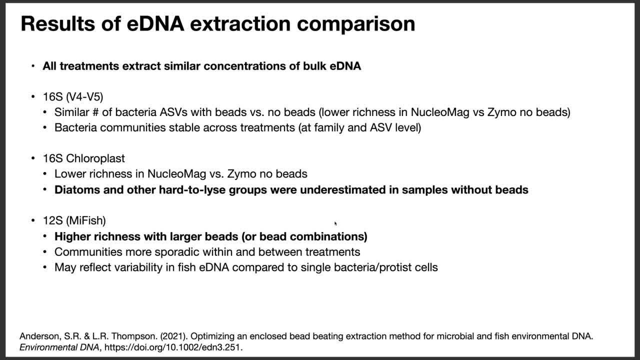 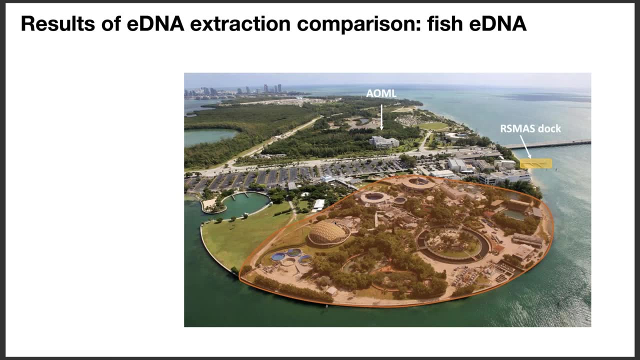 both kinds of beads, in particular was was the best, and so we recommend using both large beads, or large and small beads together, to get the highest recovery of the broadest diversity, and so an interesting thing that that happened with this survey is that we our samples were taken from the Rasmus doc, which is shown on the right there, and it's close. 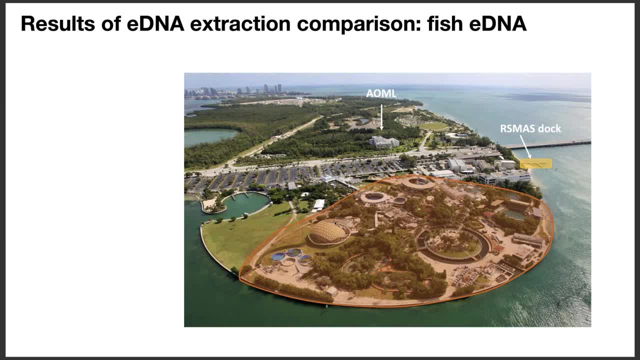 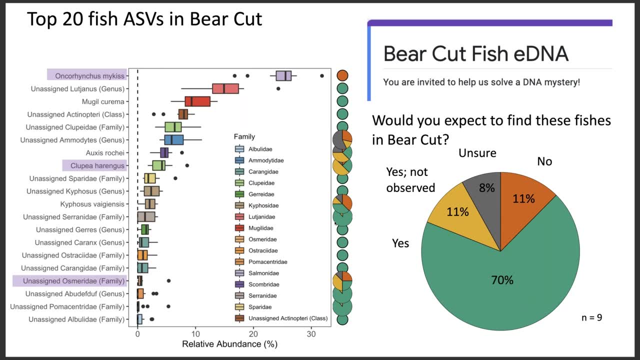 to the Miami Seaquarium on the bottom, which will become relevant in a minute, because when we looked at the sequences, we had a really interesting pattern where we saw some, saw some fish that weren't weren't expected, such as rainbow trout, herring and smelt- and make a long story short. 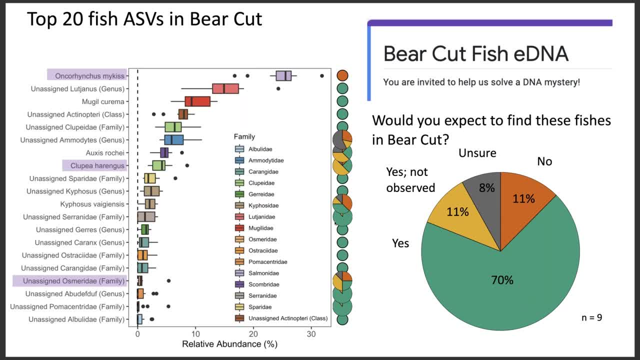 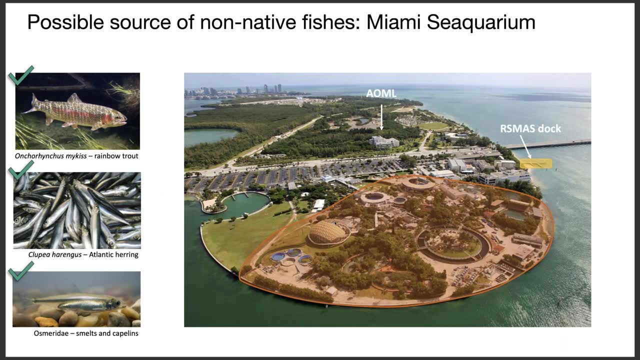 we surveyed community of local scientists and discovered that these fish were being thrown out from the, from the Seaquarium, and so these were. these were fed to their marine mammals and then the leftovers were dumped in the water and that current was going from the bottom of the screen to 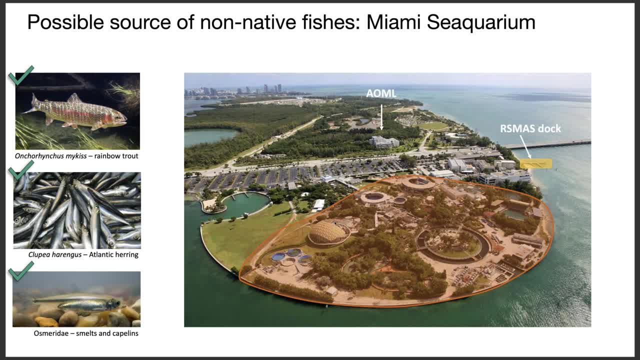 the to the right side of the screen, and we were picking up this, this environmental DNA from these fish. so it was a nice confirmation of the method, because, even though we didn't expect to see these species, we could determine that they were being put into the water directly, and so so this is a 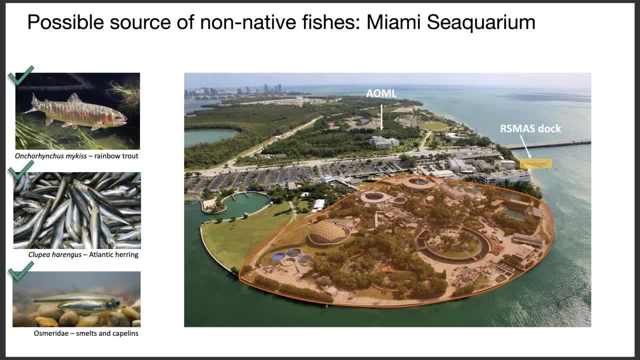 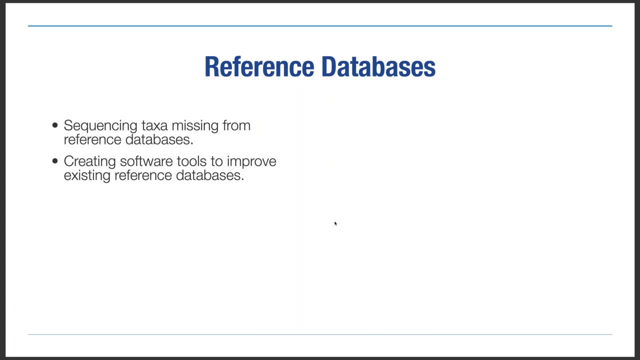 good confirmation of our fish sequencing method as well as the extraction method, which we can use in open ocean context as well as in coastal environments, and and we can use it both for collecting and analyzing fish DNA as well as microbes and plankton. so another challenge that I mentioned is reference databases, and there's there's two challenges here. 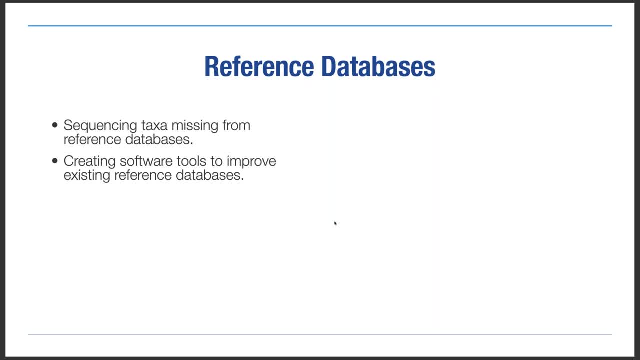 one is that we're missing taxa from some of these reference databases, and so we're we're um tackling that by sequencing taxa that are that are missing, and so we, basically, if we um we know there's something that is in the water that uh isn't in the database, that's a obviously a red flag and we. 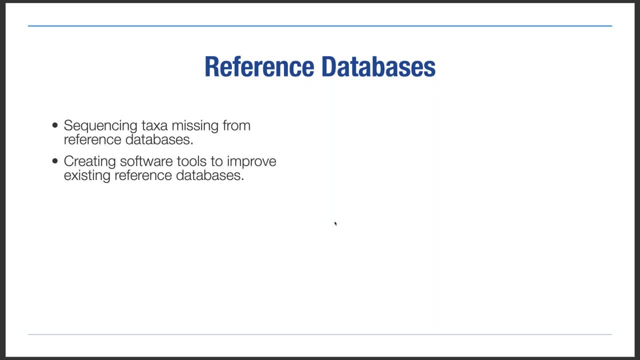 want to sequence those um, but if we also see a sequence that um is highly abundant and it doesn't match something exactly, we might be able to determine where it, where it might have come from, based on similarity, and then go ahead and target those so um. I don't have a particular slide on on sequencing missing taxa, but this is something. 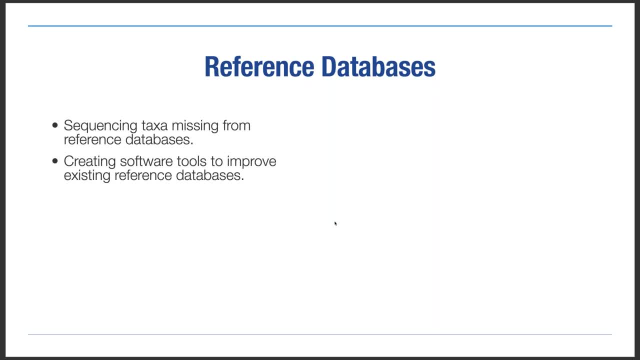 that we're working on, and the second aspect is improving the usability of reference databases that are already out there, and so this is I'll talk about our efforts on a fish specific database. but these kind of tools are are relevant to to all the different taxonomic groups, whether it's plankton, 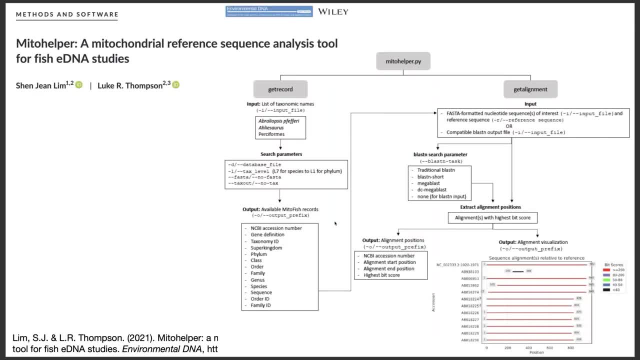 or bacteria or fish. um so um, this was led by Jean Lim in my group and she developed this tool called mito helper. um so what this does is it uses the popular um mitofish database from Japan, which is a nice database but needs some curation. it doesn't necessarily, uh, link well to the the 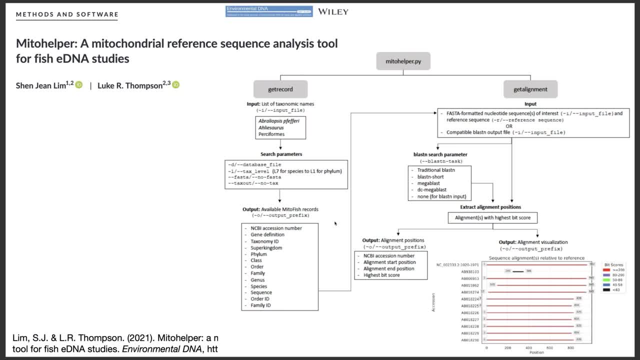 US NCBI database: um, sometimes it's unclear whether you have a a full length um reference sequence or just a part of it, or maybe the whole mito genome or anything in between. um also, uh, you sometimes want to get more information about the sequences than then. 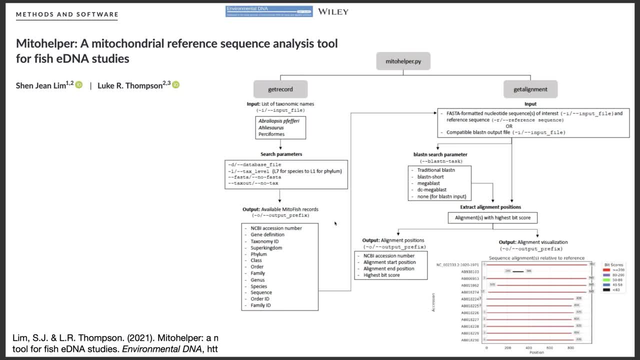 you can get. so there's a couple of different tools or commands that mitohelper provides to pull down records as well as alignments of of these reference sequences, and so this has been a, I think, a useful tool for folks and again provides it's useful for fish sequences in particular. but I think this: 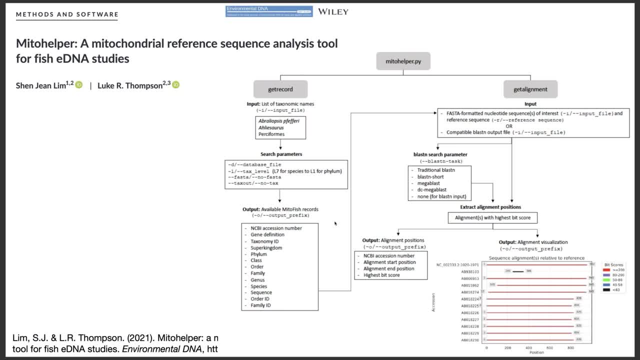 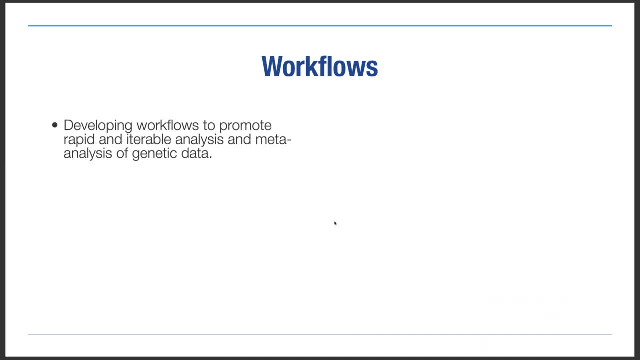 framework would be relevant to other reference databases as well. another area where we're working to improve kind of the usability of genetic data from from the ocean is developing workflows, and so this is a way to take the the kind of commands and work that you would normally do with a, with a genetic analysis of of a marine environment, and 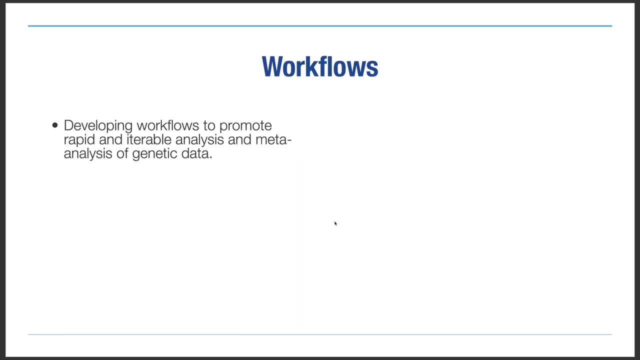 and to make those commands more rapid, to deploy, more iterable, which is to say to link between or to provide reproducible outputs. every time you run the workflow you get the same outputs that are in the same folders, you can open them the same way and you can write programs that 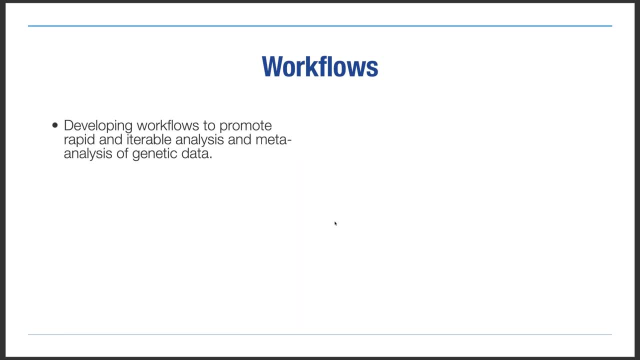 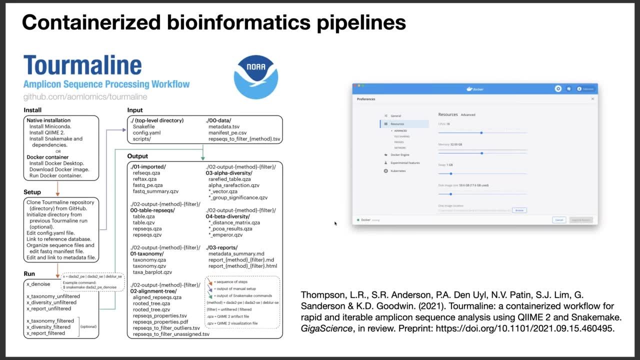 will take the output and do something with it. so everything is named for you. everything is done automatically. you can go back and change things if you want. but so we used something called snake make, which is a workflow, and what that does is basically you provide it with a configuration file, a list of your sequences or a list of your 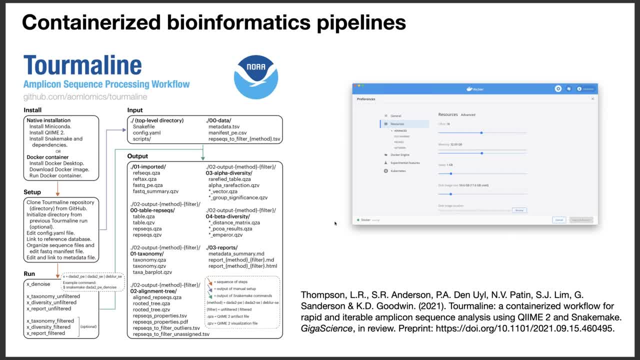 sequence files and a reference database and then it will do the rest. it will run these diversity and taxonomy and commands and then generate a report. so it's a really handy, handy tool and this is now coming out in giga science this year, so that should be 2022, but should be out in the next. 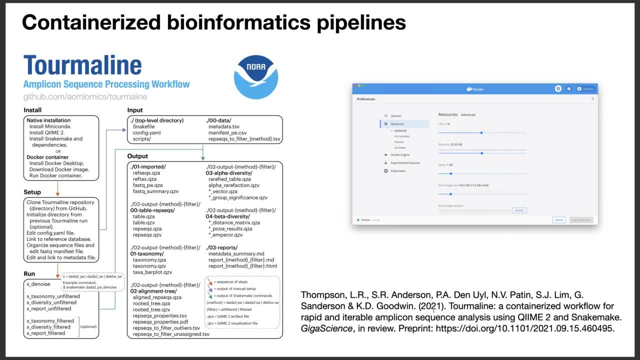 week or two. another nice feature of this, this tourmaline workflow, is that it can be run using a docker container, and so docker is a it's. you can think of it like a virtual machine or a it's a it's a system that you can you download the software, but then you can run the container and 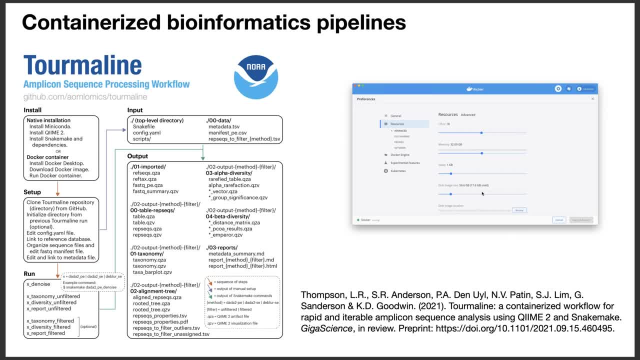 then download the container from from a server and then you can run that that container locally on any computer, whether it's a Linux, uh PC or a Mac, and and the idea is that you get the same experience, no matter what system you're working on, because you're you're working inside this virtual machine. so so, terminally comes 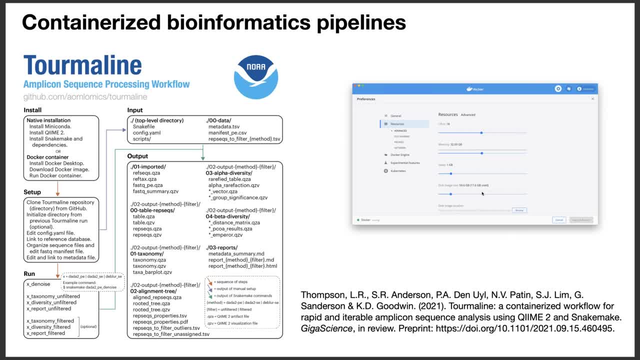 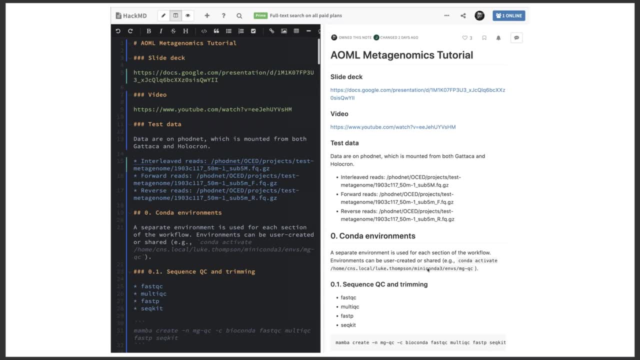 with this container that it runs inside, and so anyone can run it. you don't need to install all the software on your own computer. although you can't, it works both ways. another um sort of workflow that we're developing. it's currently more of a tutorial, but this is a 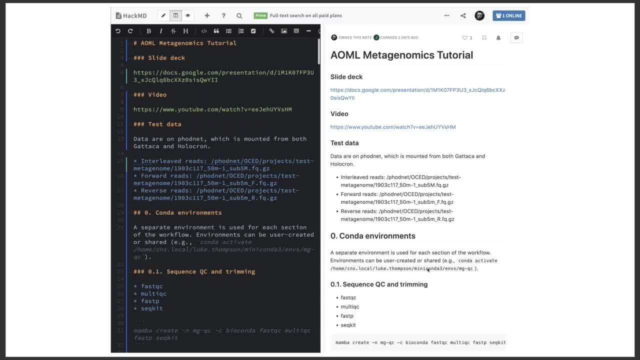 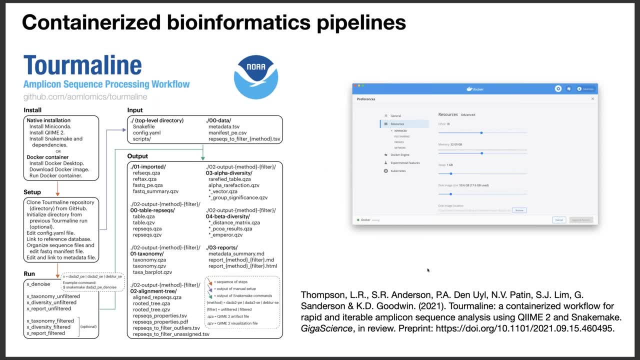 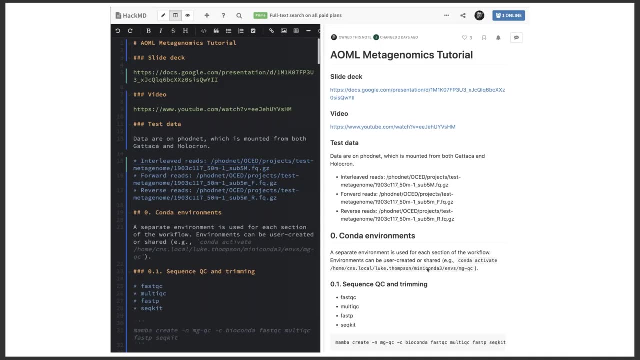 metagenomics tutorial. so the um, I don't think I said but- but tourmaline is an as an amplicon sequencing workflow or a meta bar coding. so a meta bar coding is where we sequence a single gene from all the organisms in a sample and a metagenomics is where we we sequence all the DNA. 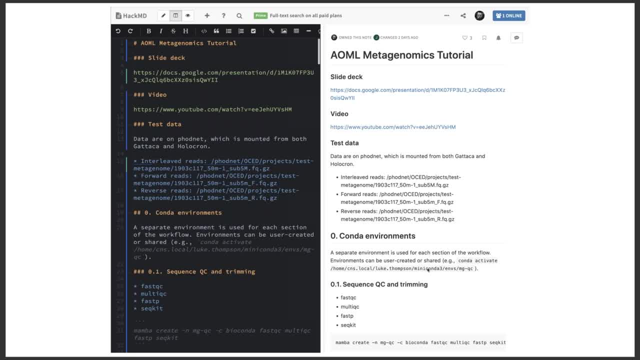 from everything. so it's. it's a more complicated analysis, but um, Nastassia Patton and our group at aoml have been developing a metagenomics tutorial, that work that walks the user through um, through an analysis, and um and Nastassia gave a great presentation a few months ago and- and there's 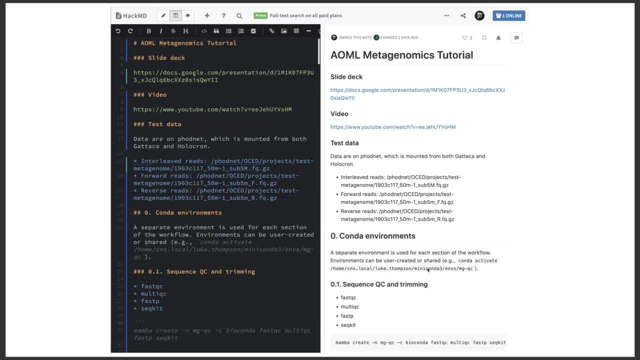 a video recorded of it, so she really provided the background for how you do this. and then we've put the commands and uh instructions in a single Markdown document and we're working on this now, and and the idea is that it'll be both a tutorial for people to learn metagenomics, but also, potentially we can turn this. 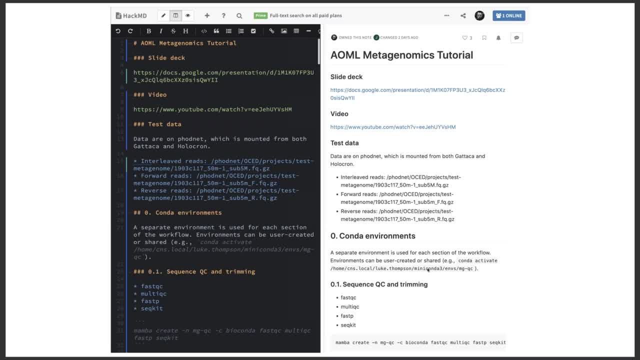 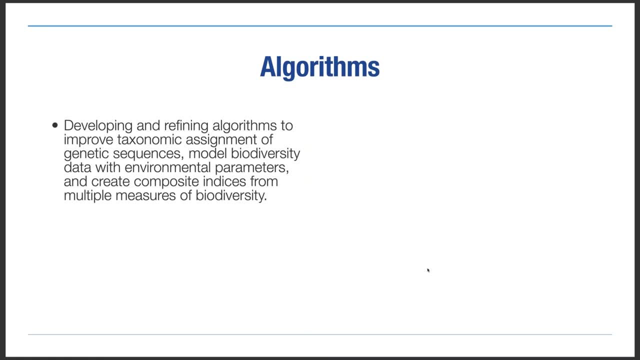 into a workflow as well, so you can actually run it on your, on your samples, and then another um technical thing that we're we're developing are algorithms to um, to improve taxonomic assignment of sequences, um, as well as to model biodiversity with environmental parameters, and eventually we 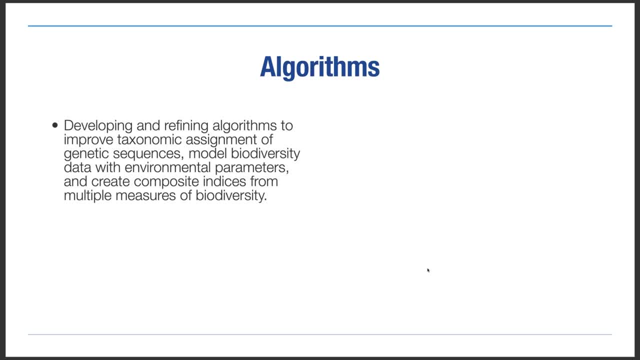 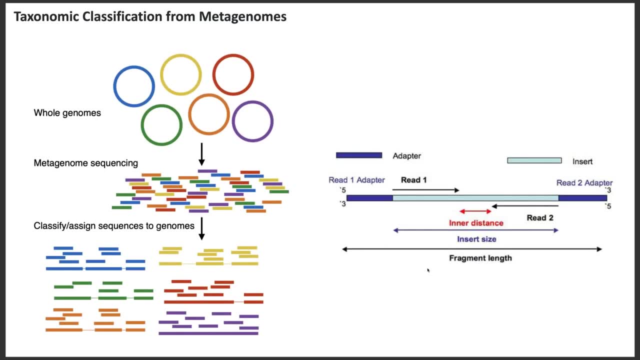 want to create composite indices from multiple measures of biodiversity. so, um getting started, we've been working on some machine learning algorithms for taxonomic classification from metagenomes. so um this kind of would fit into that. um that tutorial I just mentioned on metagenomics, um part of analysis of metagenomes is to figure out what are the the taxonomic groups in that sample. 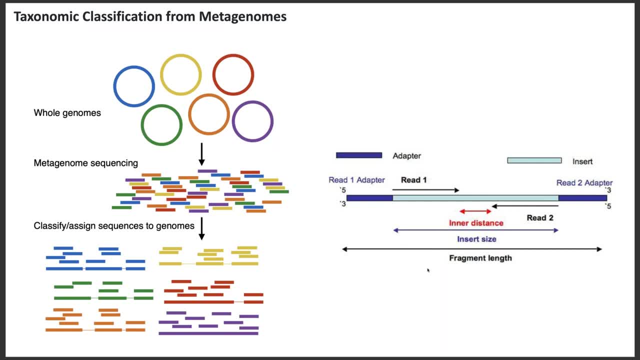 and so, um what? what we've done- and this has been um led by Gene Lim in my group- is to: um, well, when you do sequencing of, of of microbes in particular, you can think of each microbe um having a genome represented by a different colored circle, so you chop up the DNA and then 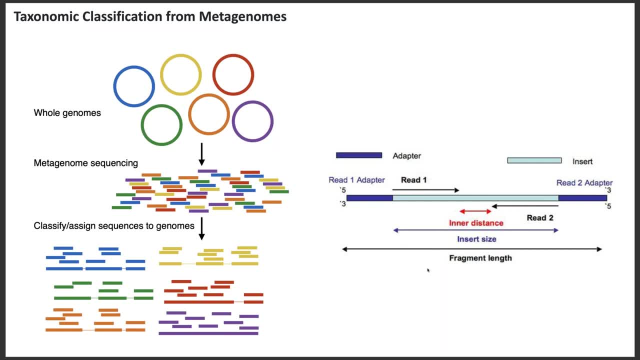 um, you align them and and or otherwise classify them, try to figure out which microbe they came from by comparing them to reference databases in in some way or another, but there's lots of different ways to do that. so, um, uh, and, and I've included this figure on the right which shows: 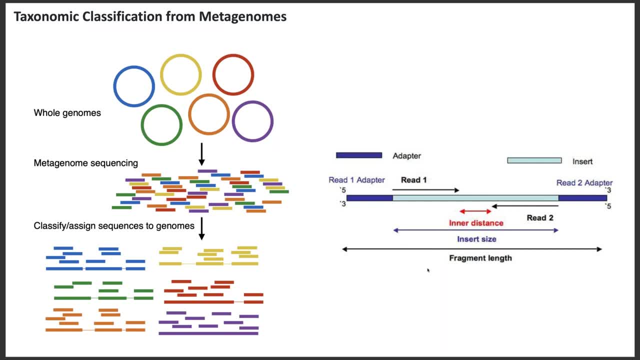 that when you have a sequence of DNA- um, you typically- or a piece of DNA, you typically sequence the two ends of it, and then you have some part in the middle that's unsequenced. so this is called paired end sequencing, and so when we are trying to classify our sequences, we have to deal with that. 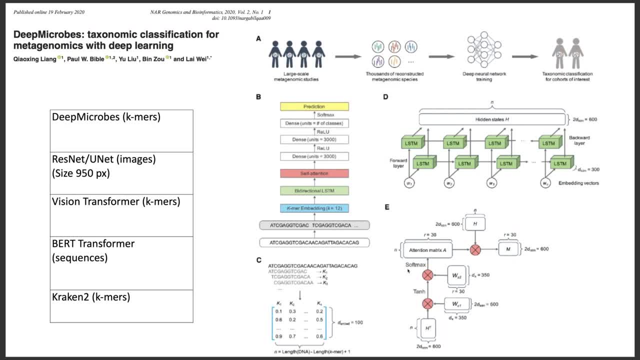 so what? what we've done is we've been using this algorithm called deep microbes, and this is a taxonomic classification algorithm that uses some deep learning methods, such as long short-term memory and including deep neural network training, and also uses a k-mer based approach, which is where you 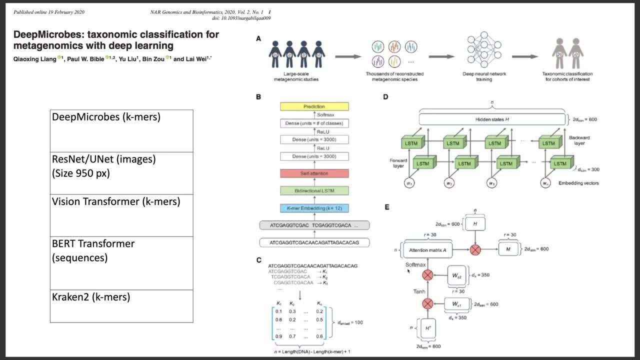 break up the sequence into lots of different pieces. so gene and an intern working with us, Helen park, have been testing this out, training this algorithm or training this model using marine metagenomes, because this is a part of the engineering process we've had over time. program was developed for gut metagenome, so she's helen and gene are using this with marine. 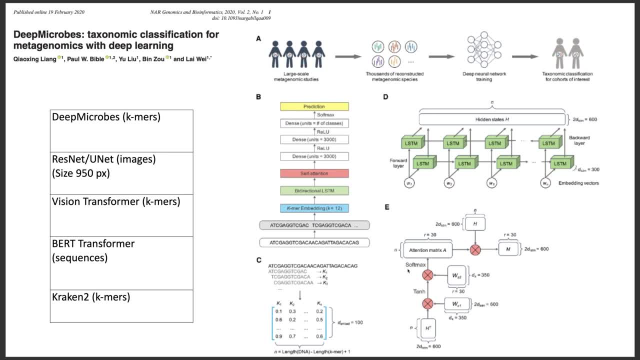 metagenomes and then training the model and then testing it on different data sets. meanwhile, we've got a group of of researchers that that was organized around an nvidia hackathon back in february and this group has continued to meet and we've got several different algorithms that the 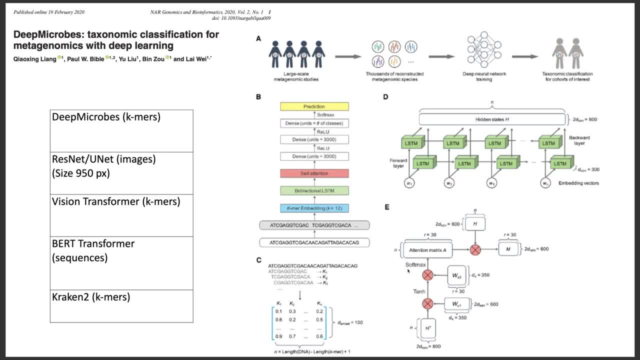 group came up with using various machine learning algorithms, one based on images, another based on gamers, which are those short sequences of letters. another based on the bert transformation, which is what like google uses to to suggest, like, what's the next word? you're going to type that sort of thing and then we're comparing that to a standard. 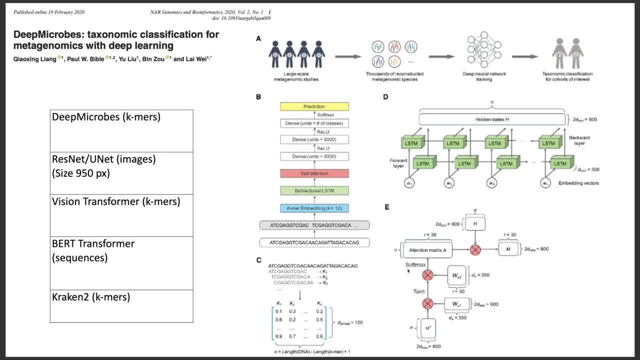 data base, like using a full database and camera based approach, a method called kraken2, and so we have some, some different algorithms that we're comparing, and so the end goal of this is hopefully that we'll have multiple methods for for analyzing or determining the taxonomic. 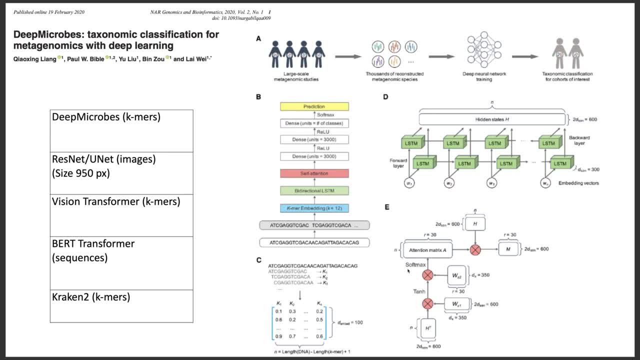 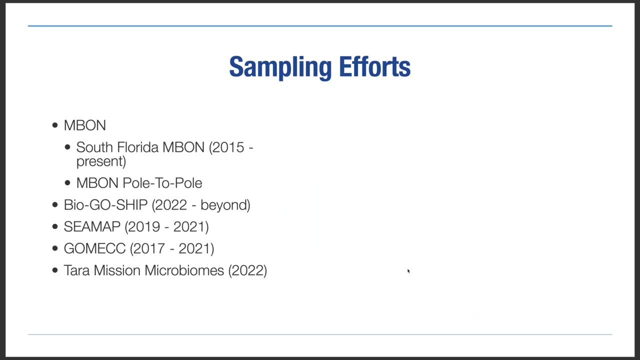 composition of a microbial samples from the ocean and potentially a better algorithm. in some cases that might improve on existing existing technologies. and so now i wanted to turn to some of those sampling efforts where we're we're going to start applying. you know, eventually, when we get sequence data, we'll start applying. 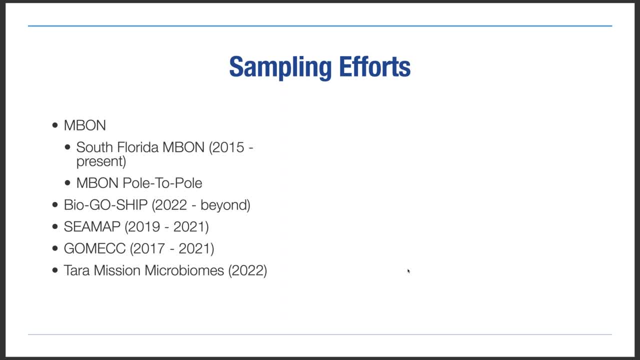 those, those methods, um to these surveys and that are going to give us a wider view of the ocean, and i'll talk a little bit about what comes next and what we're going to do in the next couple of weeks, in a little bit longer, and then we're going to talk about what kind of information we can get from. 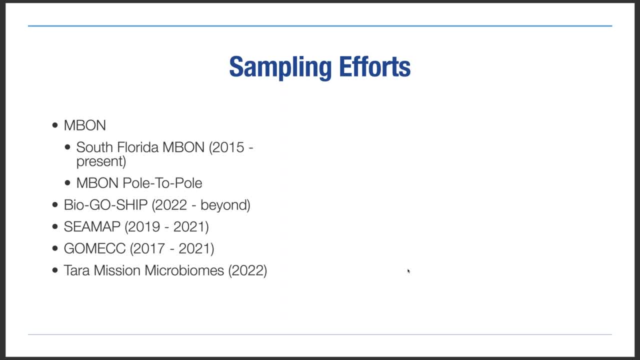 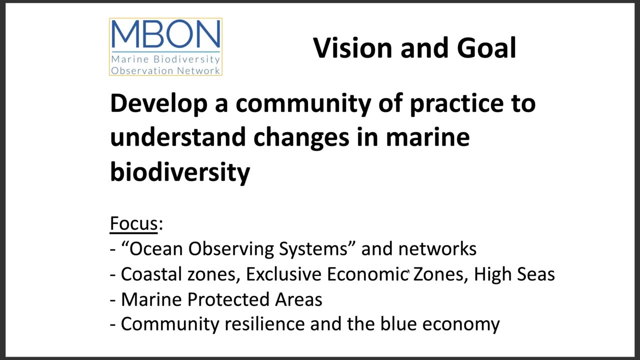 those surveys and then i'll i'll conclude with some um, some results closer to home, from the gulf of mexico, where we're a little bit further along in doing some of this work. so, first of all, mbon, the marine biodiversity observation network, the. the goal of of mbon, or the vision, is to develop a community practice to understand. 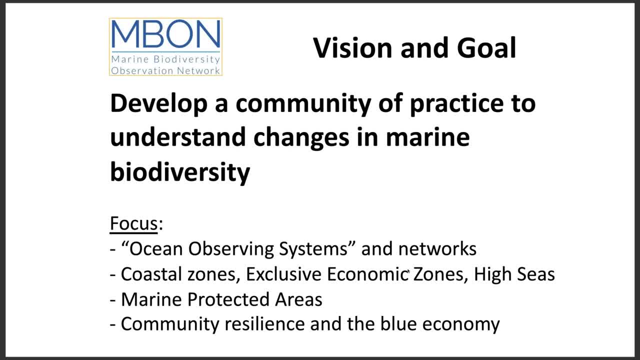 changes in marine biodiversity. so it's the idea is ocean observation, um systems and networks of different groups and scientists around the globe, both coastal EEZ and the high seas, so everything is fair game. There's a focus on marine protected areas and then focus on community resilience in the 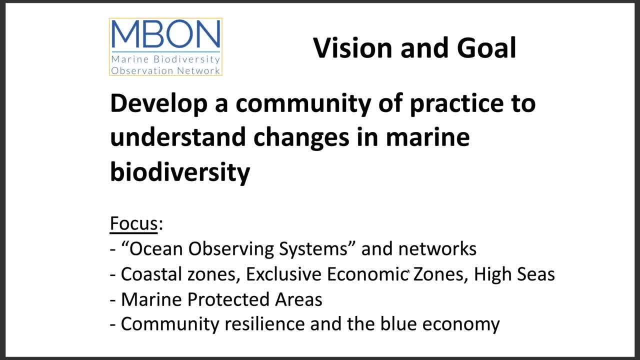 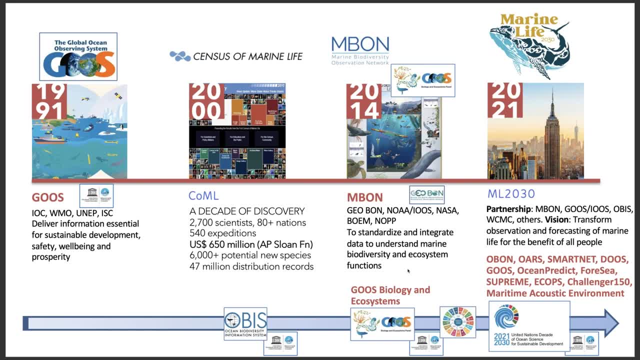 blue economy. so there's a, you know, an economic component to this as well, And so MBON has been around for a while, and it's continued to grow over the last few decades, to the point now where there's a lot of buy-in from the United. 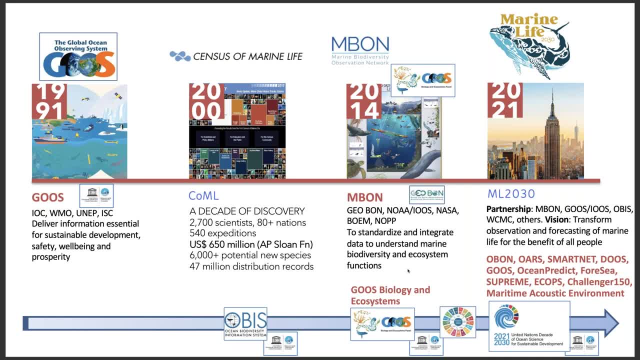 Nations from different organizations. One that I wanted to mention was OBON, which is the OMICS Biodiversity Observation Network. We also have GOOS, IOOS, involvement from BOEM, GEOBON, NASA, and so it's a, it's definitely a. widely, there's a lot of. 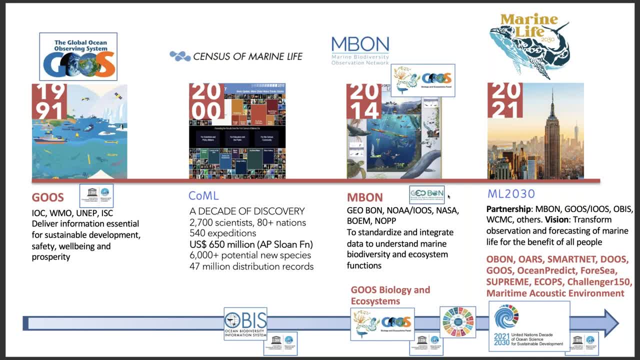 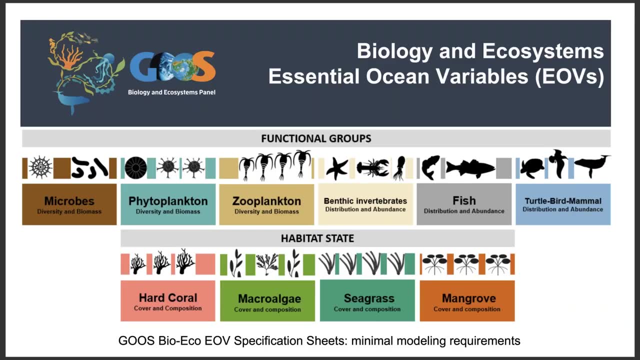 buy-in a lot of participation across these different communities and so, and especially with the UN decade happening now, it's an exciting time to really really spark these collaborations. So one aspect of MBON is the use of these GOOS- biology and ecosystem essential ocean variables, or EOVs. so 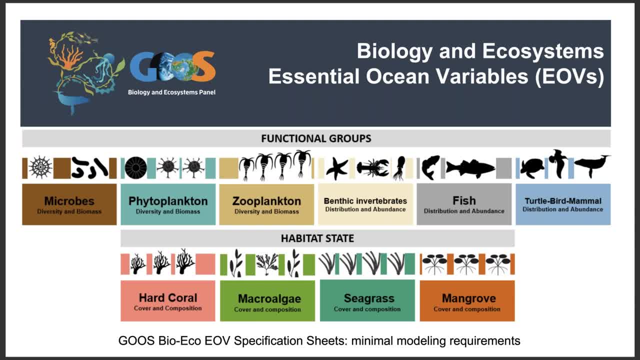 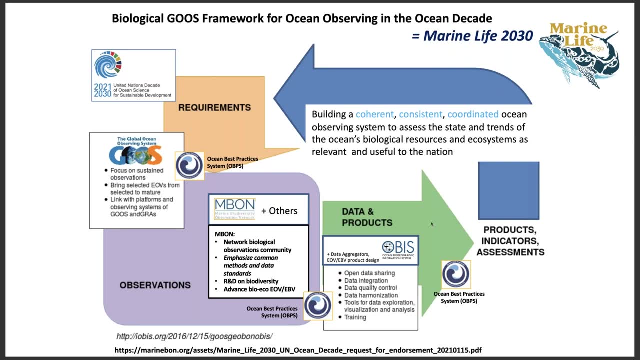 there's a variety of different functional groups or different taxonomic groups, as well as different habitats that are, that are focused, focused upon, And so the the way that that this observing network is meant to to work is where we kind of have a feedback, where we have 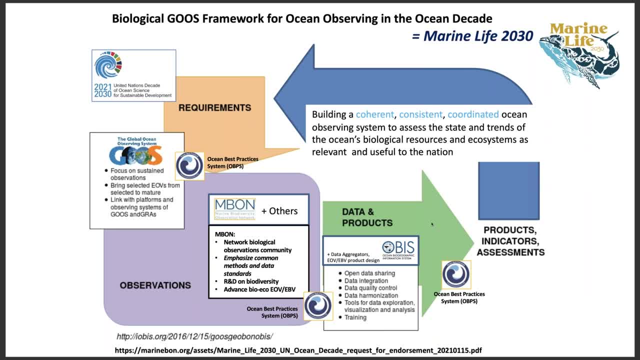 requirements for how observations are made and reported as observations are made, which leads to data products and and sharing across, across different communities and end-users and and stakeholders, And that then builds this coherent, consistent and coordinated ocean observing system, which then feeds. 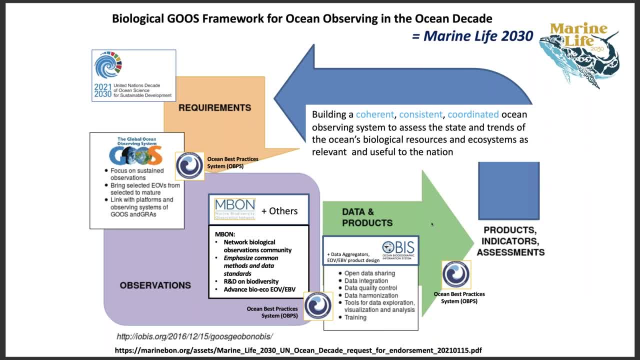 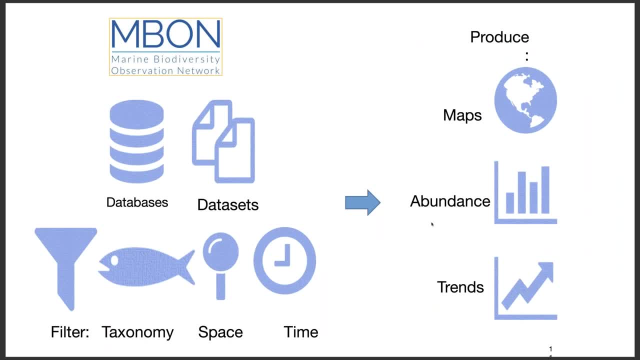 back and improves requirements and improves the network and improves the next round of observations. um. so put another way, um, from the data and data sets that we? um that we collect and we can, we can slice those or filter them by taxonomy or space or time we get. 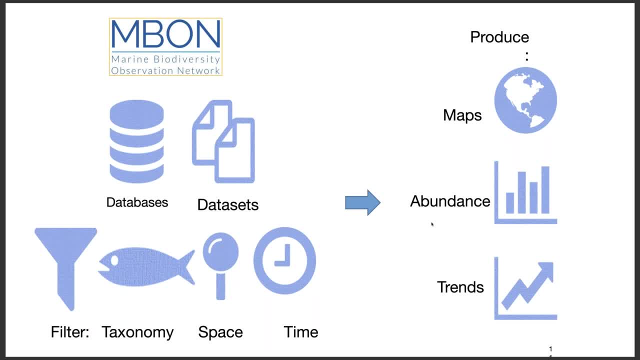 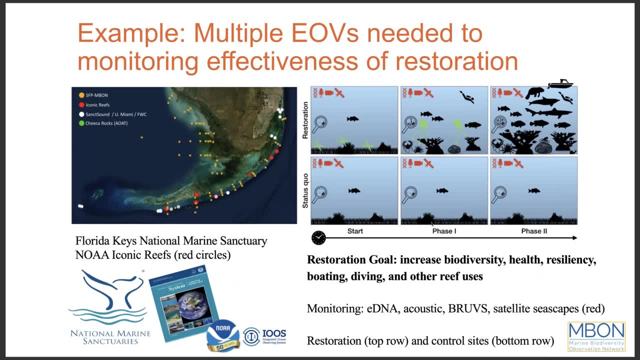 maps of abundance and as well, we can graph trends and see how things are changing over time. um and so an example of of these um of mbon, uh, would be the the south florida mbon. so this is um the south florida mbon. stations are shown in the map in orange. 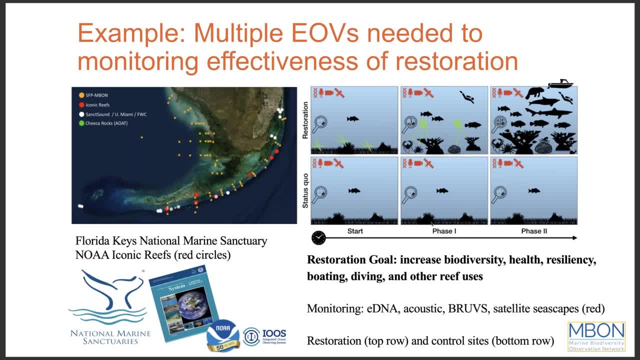 but they're very close to the noaa iconic reef sites, where there are some reef restoration as well as a couple other sampling efforts shown on the map, and so one of the things we're starting to do is um is sample at these sites, in particular, the iconic. 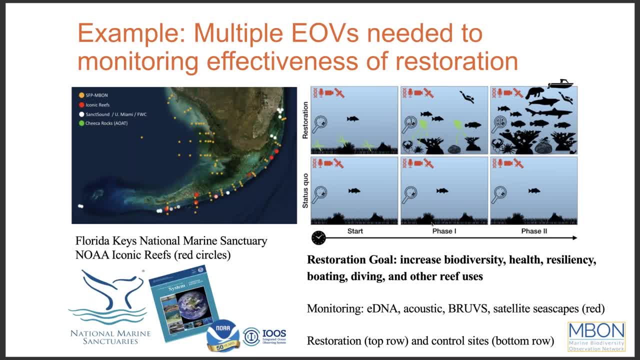 reef sites um over time, uh to to determine, um you know, how the the reef environment is changing and and how the biodiversity is changing as we restore reefs um, and so one of the things we're doing um is um using um edna uh, as well as. 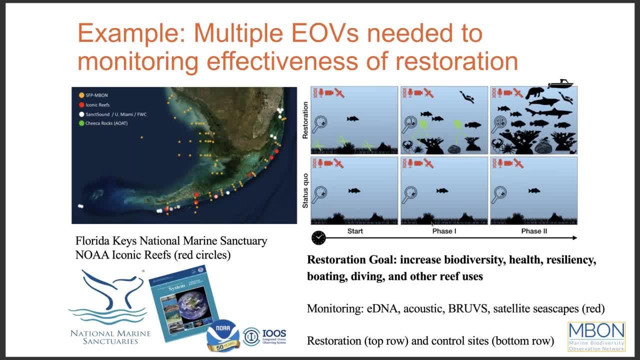 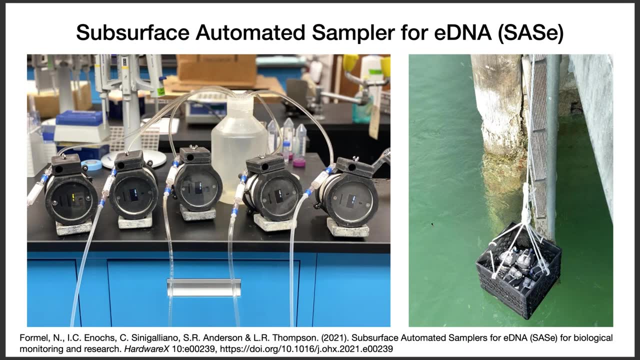 satellite remote sensing to monitor those changes um, and so we've started this, this project. now, um we've got some, some seed funding to do um edna sampling on reefs, and so we're using the um subsurface automated sampler for edna or sassy that was developed um by nate formel and ian enox. 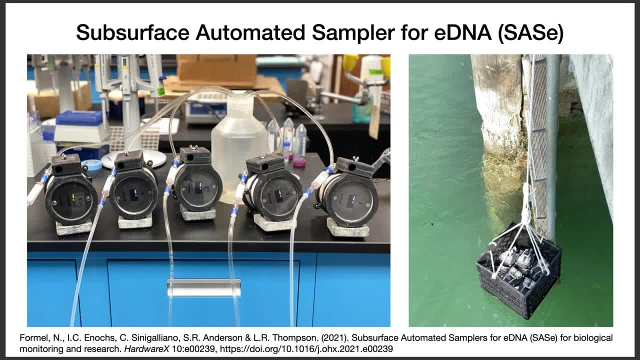 at aoml and um. so this is a little peristaltic pump. uh, that holds one of those starevex filters i talked about earlier, um. so actually this afternoon we're doing, um, one of our first pilot experiments in the field, um and uh. our hope is that we can get these working. 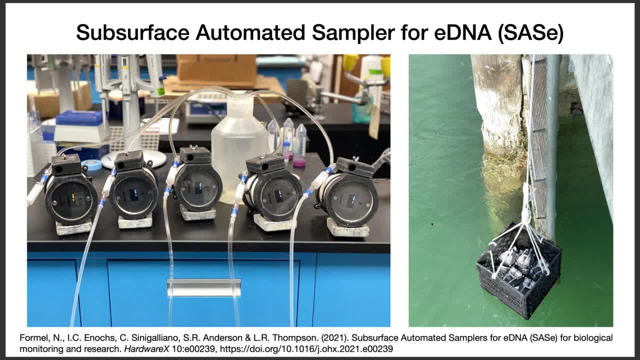 um, you know they work fine now, but we haven't done a lot of testing in the environment. so get them environment tested, get some data back and then by next year we'll be ready to do some sampling on the iconic reef sites and start to monitor, um monitor how the community of fish and invertebrates is changing with restoration. 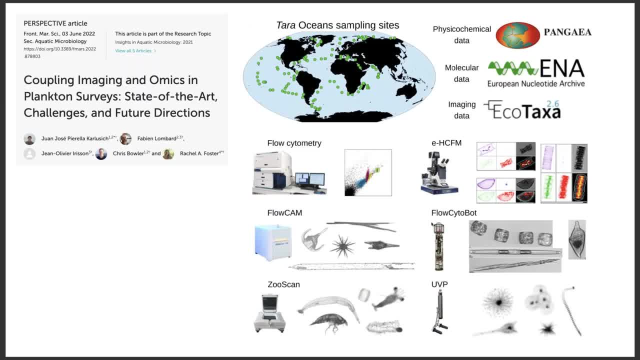 and then i want to talk about um biogoship. so, um, before i talk about biogoship specifically, i want to talk about a related effort that i think is is really important to um, to think about what's possible with biogoship. so, um, this is uh related to the tara oceans, um, 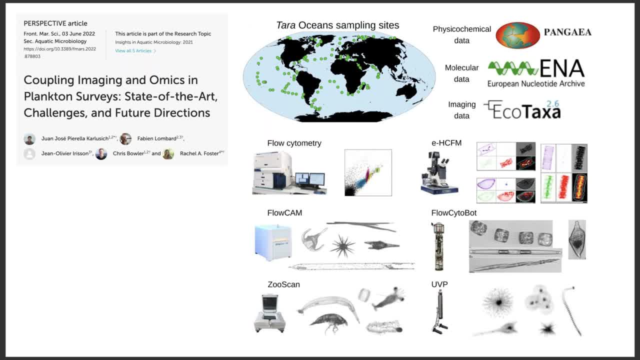 so um. tara oceans is a a french um and european-led effort to to monitor biodiversity around the ocean using a lot of technology, a lot of different imaging, as well as genomics methods and so um. this is a a figure from a paper um published by by some of the tara people. 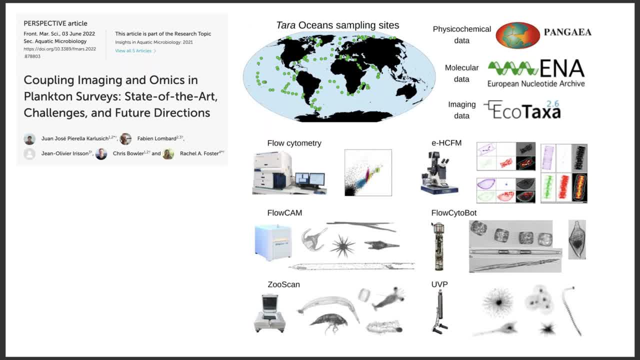 um in frontiers and it's about coupling imaging and omics in plankton surveys. so from these different tara sites they have a ton of data um various different imaging methods and that that target different um size fractions of plankton um as well as the the omics part of it. so 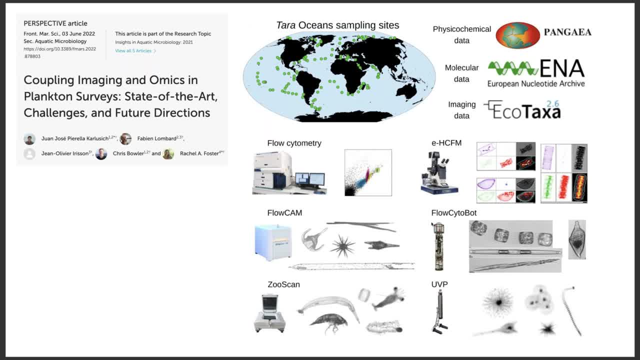 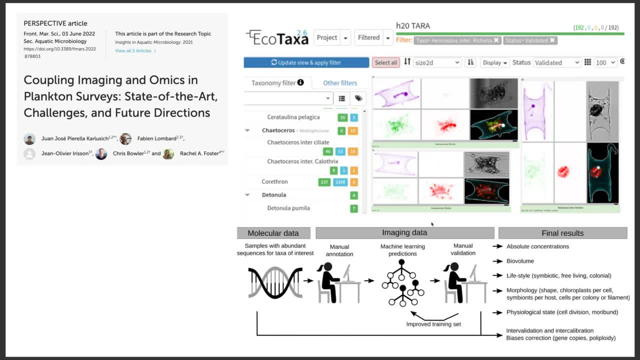 um. so they've- they've really done some, some cool stuff with this, with this data. so, um, one of the things they developed is this ecotaxa program that allows them to annotate the imagery um and then they can validate that with um genetic data. so there's a lot of. 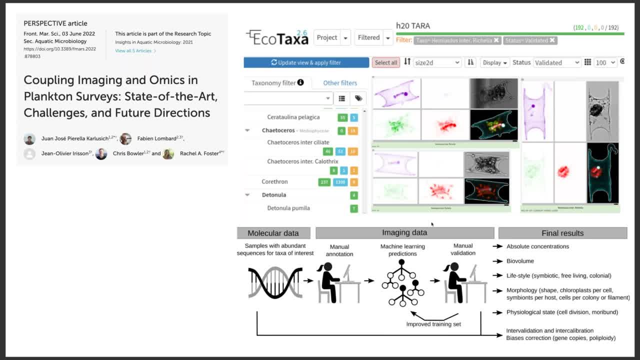 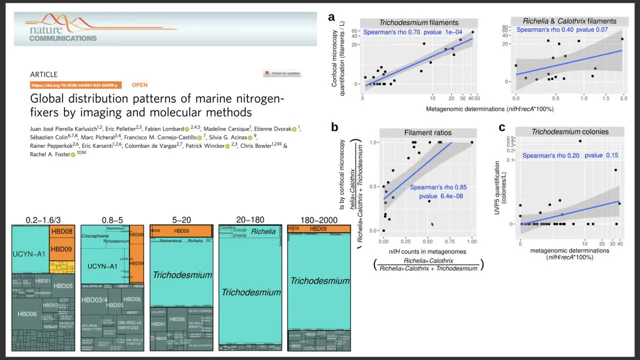 technology that goes into this, and um, so they've- they've used this to do some some cool stuff. so, um, they had a paper out um last year, i believe, in nature communications, where they were, they they analyzed just a ton of data from all these different stations and so on. the lower 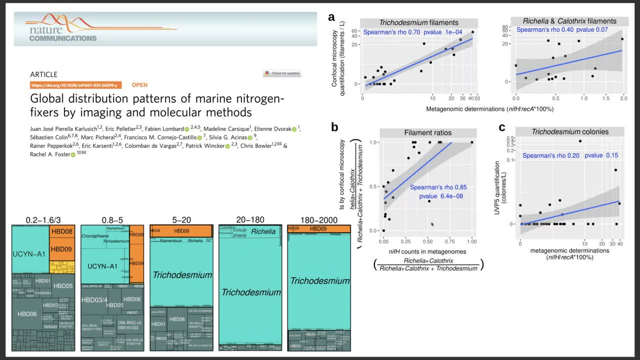 left is showing you um using the omics method, the uh, different uh, so that they pulled out and the ones that are colored they could identify um. so there's some different um. in particular, this is focused on um diazo tropes or or nitrogen fixing, plankton, and then they com, they compared uh. on the right, they compared the um, the relative. 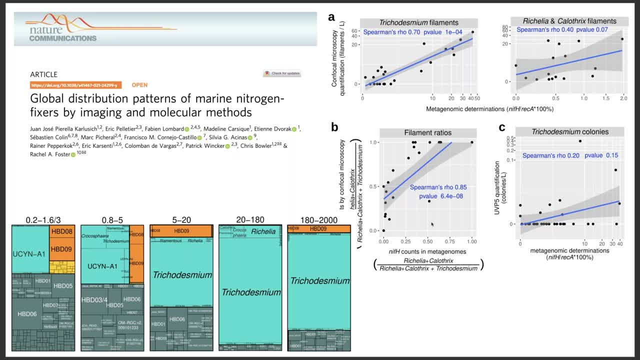 abundance from the, the genomic methods, versus the amount relative abundance with the imaging methods and um. you know they're not perfectly aligned but there's there's some good um overlap and so they're. they're showing that you know these two methods are, are both, um, you know, effective. 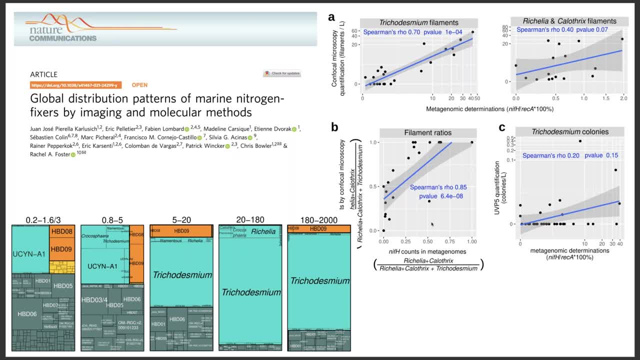 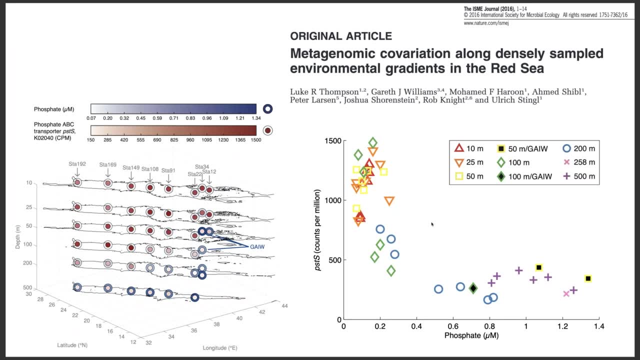 and complementary to getting a fuller picture of of plankton in the in the ocean. um, switching gears a little bit um. another uh thing you can do with marine omics or marine genomics is you can the relationship between nutrient levels and the genetic functions that are involved in those. 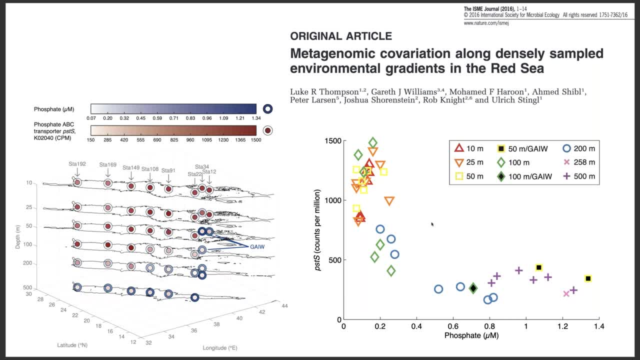 nutrients. so this is a paper that i wrote several years ago from some data in the red sea. so on the on the right is a kind of a contour map down the water column of the red sea from the surface to 500 meters, and each of those circles or concentric circles, is a is a sample where we took environmental 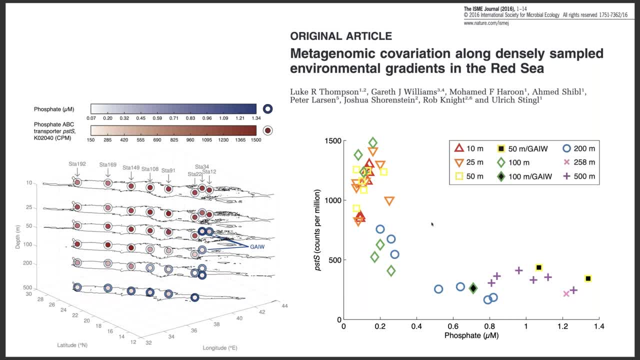 metadata like nutrients as well as metagenomes, and then the. the colors show um, on the outer circle the phosphate concentration and on the inner circle, the the sort of relative abundance of the phosphate transporter, uh, the gene for the phosphate transporter, psts. so what it shows is that there's an inverse relationship between the phosphate concentration. 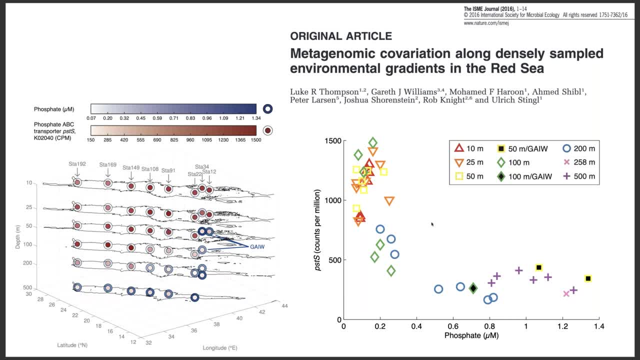 and the likelihood of microbes having the gene for transporting phosphate. so when phosphate is low, microbes are more likely to have this transporter because they need it to transport. phosphate is the hypothesis, whereas when phosphate is high, the the need for this, like high affinity transporter, is not as much. and the same information is shown on the right, just in a, in a. 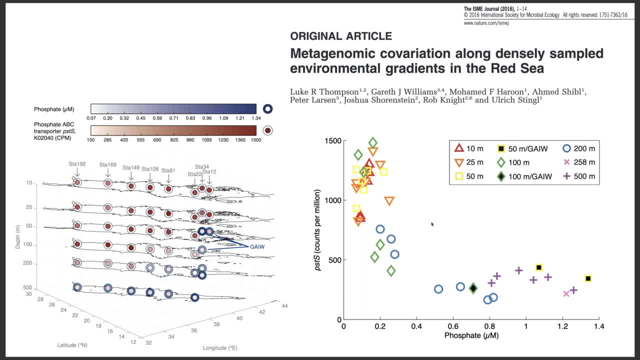 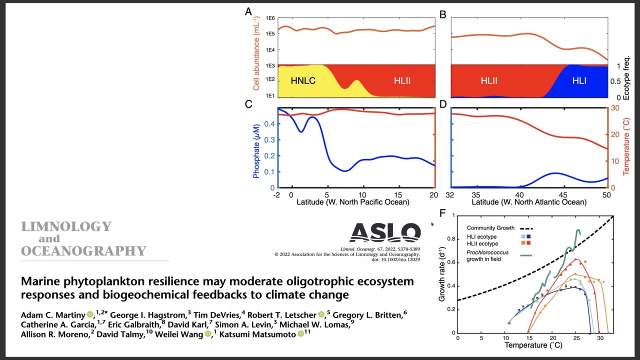 graph form and so the very clear relationship between um phosphate and this, this gene. so this is a single example, um. but then adam martini's group at uc irvine, and adam is a um, a collaborator on the biogoship project- they've sort of expanded this idea to look at. 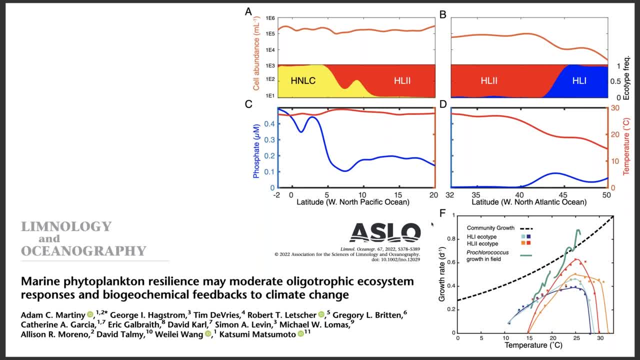 um, in this case it's looking at prochlorococcus across the global ocean. um so so. on the graph here you can see um latitude in the pacific and then in the atlantic, and there's these really striking trends of phosphate concentrations and then ecotypes. 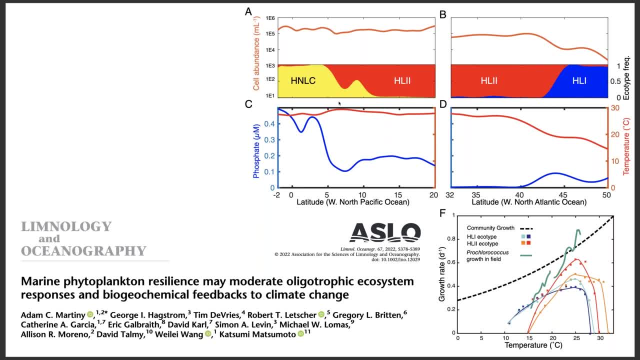 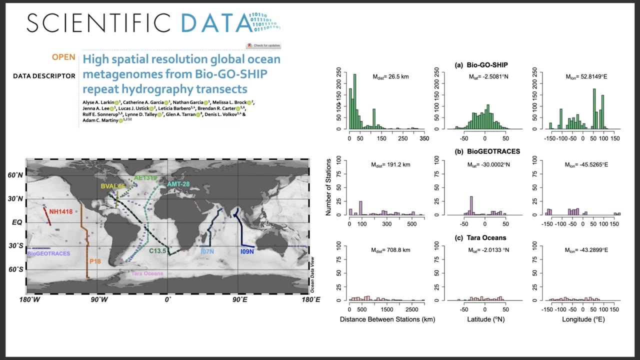 or or kind of groups of prochlorococcus that that correlate really well with phosphate as well as temperature, and so, um, there's a lot you can do with these ocean transects, like we want to do in, like we're doing in biogoship, and so, um, what adam's group also did was they took, uh, some goship. 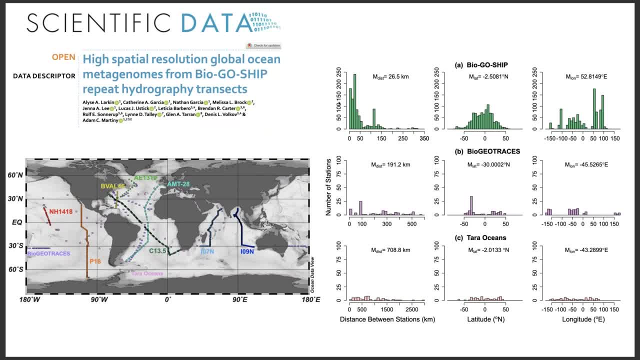 um, i think they did one or two, yeah a couple of of goship lines, maybe three uh, p18 and i07 and 09- um they did those biogoship um lines and they also got samples from biogeotraces as well as tara. 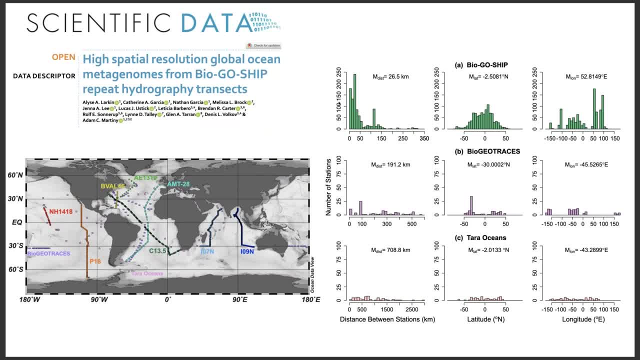 that i just talked about, and they sequenced metagenomes from those um, and so one of the things that you can see um in this um graph on the right is that the, the resolution of biogoship, is much greater because of the way the sampling is done, and we can sample continuously. 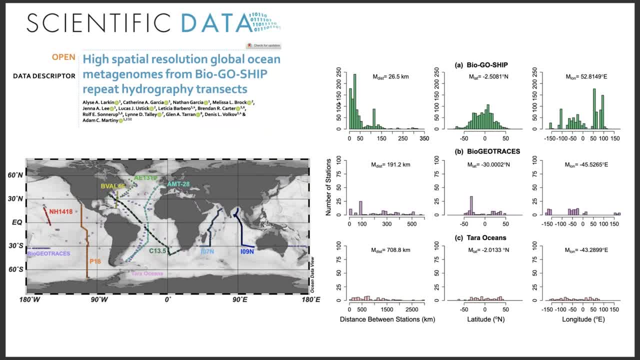 kind of you know, every few hours as the ship is going um, we can just get water from the ship's flow through system. we can get a lot higher resolution um in biogoship than we can in some of these other operations. maybe we don't get quite the abundance of different kinds of data but we 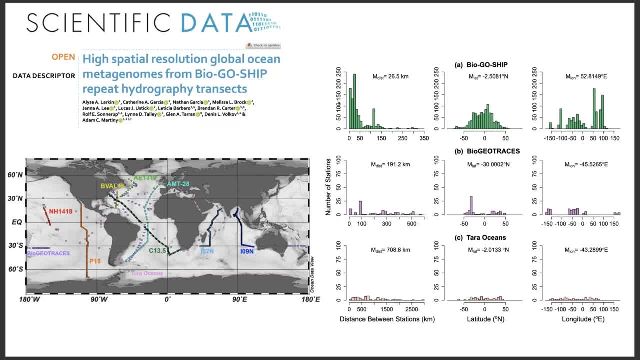 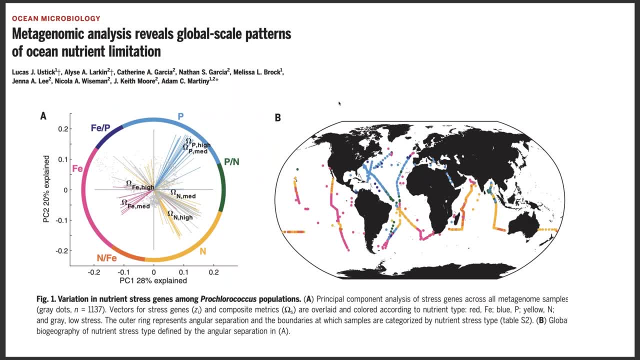 can get a lot better resolution, which which provides opportunity for some cool um analysis. so so adam's group then took that data and they had this really nice paper in science where they were able to determine um, the nutrient, uh limitation regimes of different parts of the ocean. so these 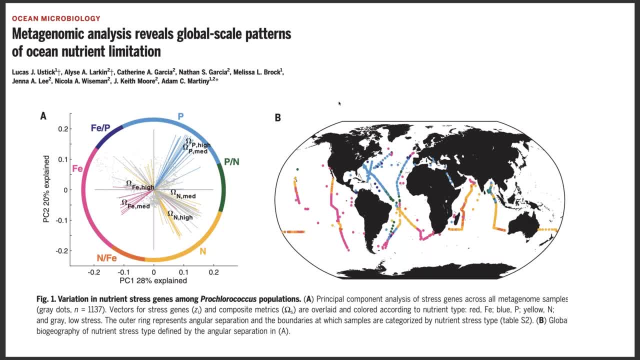 lines shown in the map on the right are those same lines that i just showed you, but now they're colored by um, whether, uh, the, the microbes, and it's based on these genetic um, these genetic um measures, like i showed, from the red sea, which um samples are. 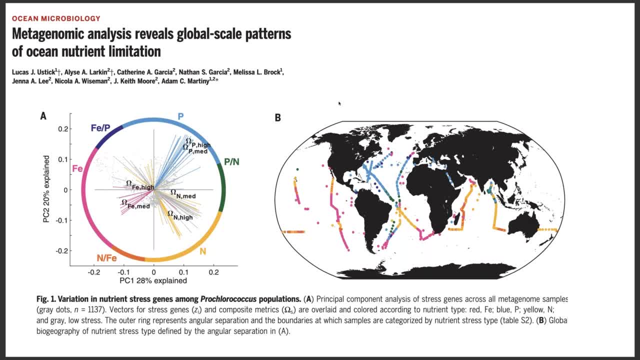 are nitrogen limited or co-limited, nitrogen and iron or nitrogen and phosphorus or phosphorus limited or iron limited or iron and phosphorus. so this is the kind of thing that's only possible with um, with global sampling of the scale, um, you know, like gosha. 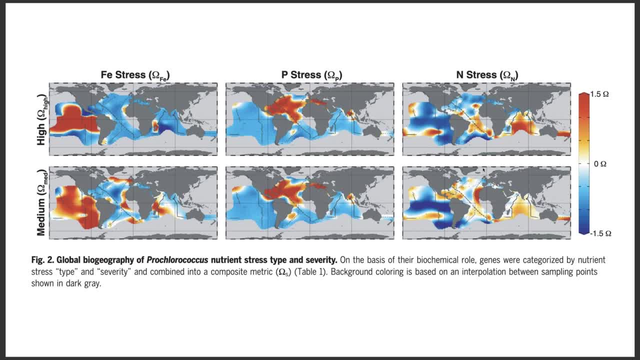 and then, uh, just another um way to look at it is: you know, you can look at the map and and, based on what we know about um parts of the ocean that weren't sampled, we can extrapolate. um, you know which parts of the ocean are under iron stress, phosphorus dress or nitrogen stress? 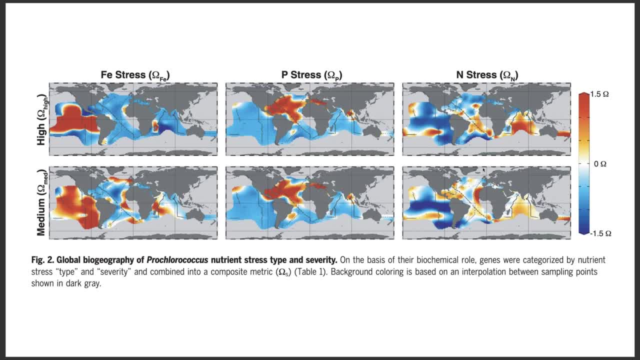 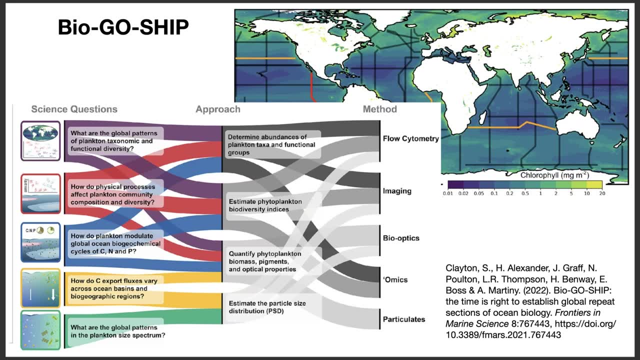 and then of course there's some co-limitation in certain parts where those regions overlap um. so with biogoship, um we we want to expand this. so, um, my map got covered a little bit, but there's around 66 lines in the goship program, um, with the, the biogoship pilot, um we've got um three or four. 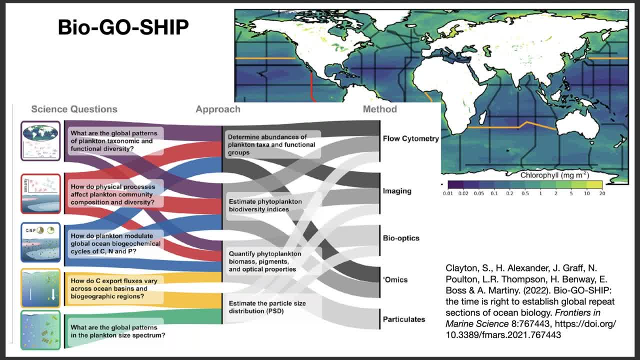 lines that we're going to do um and in addition to metagenomic sequencing, like like adam did um with those other cruises, we're going to add a variety of imaging methods, similar to what what the tara group is doing, and that allows us to to combine these different methods and really um new ways to 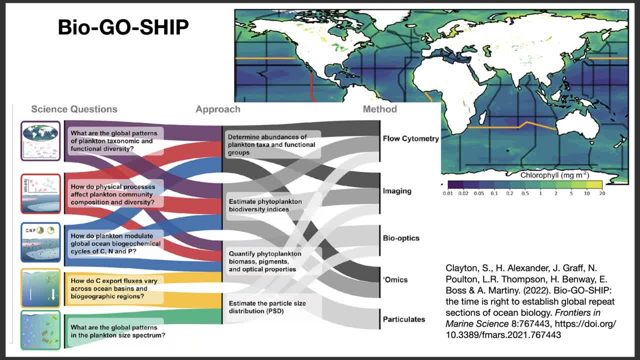 to look at relationships between these genomic measures as well, with um things like particle size, optical properties, um phytoplankton abundances and diversity, and and then come up with, based on all that data, come up with um models and and indices of of diversity and how um. 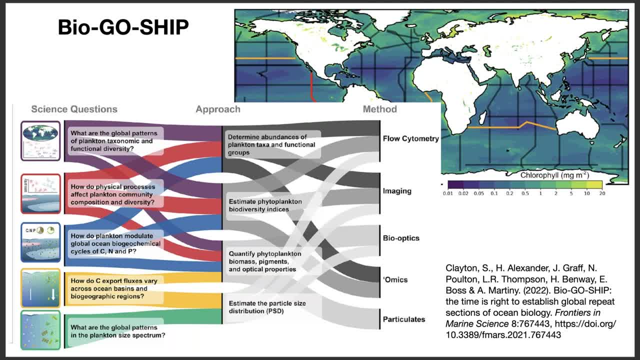 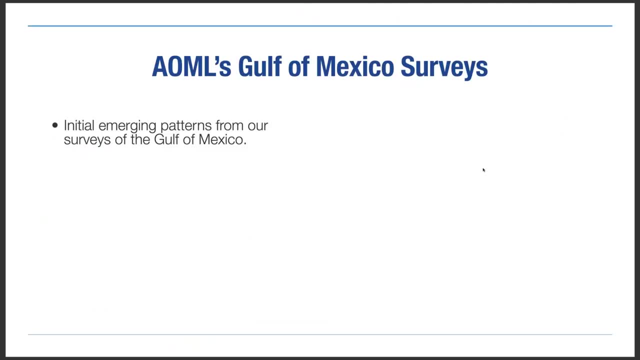 i think, come up with ways of representing that diversity in um using multiple metrics, that's that'll be more sort of more powerful, more robust and more informative for um for things like conservation and modeling. and so, finally, i wanted to talk a little bit about um some 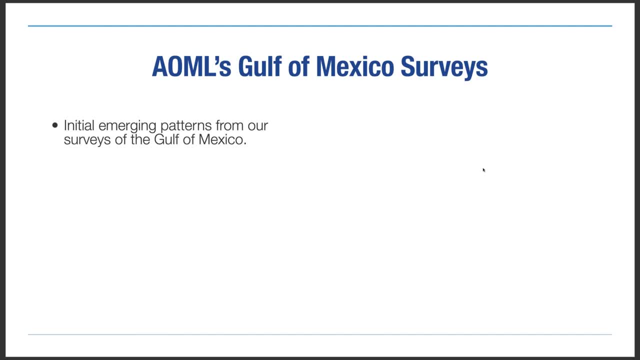 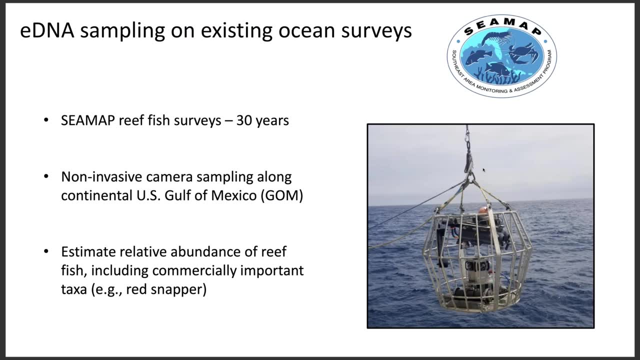 of the other things that we can do to help us get closer to home. um, um, looking at the gulf of mexico and and what we can, uh can say about, uh, some of the patterns we're seeing here. um so this one is from the? um, the southeast area monitoring and assessment program, or cmap. um so this is a. 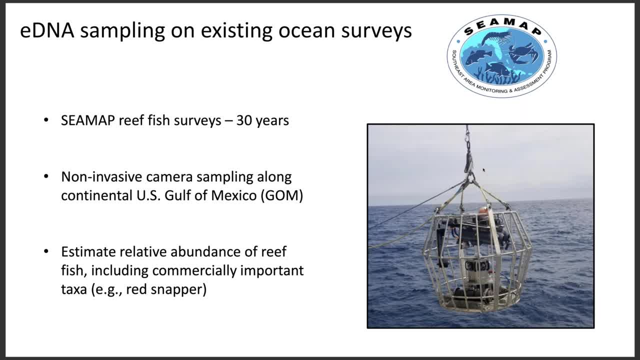 survey that's been going on for 30 years, um, and, and they're using um camera traps, like shown in the picture there. so when, um this, uh, these bottles are closed while the camera trap is down on the sea floor, um, so it's, it's taking video of fish to swim by and then we can um close those those bottles and we can measure both. 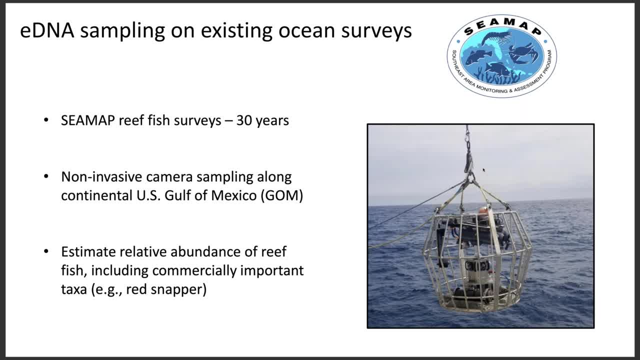 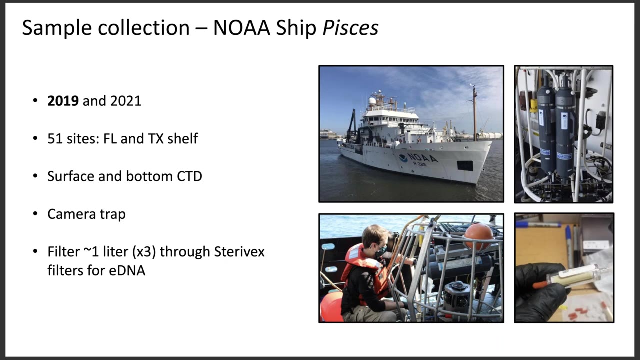 fishy dna as well as um, plankton and microbial uh dna to get a picture of both um. you know how well the fish compare to what's in the, the, those bottles, as well as um. that's how that relates to the, the lower trophic levels, um. so uh, we are still uh getting the last of our data sequenced from. 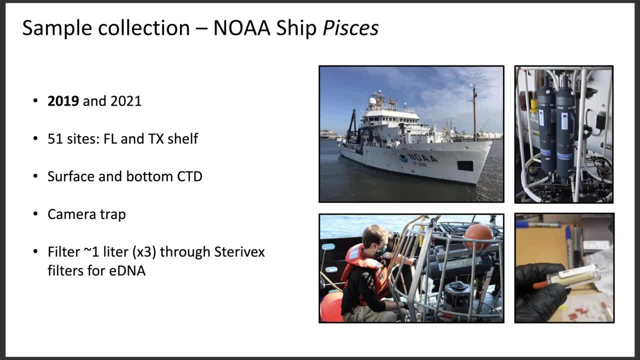 2021 um. so what i'll talk about today is is um the data that sean has analyzed from 2019 um. we've got sites from florida and the texas shelf um surface and bottom um using the ctv um, and these were all sampled using that sterebex um. 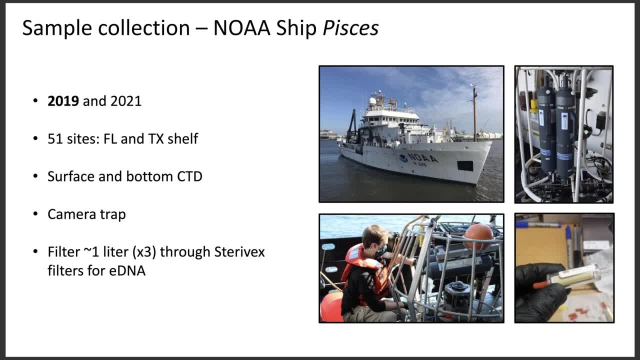 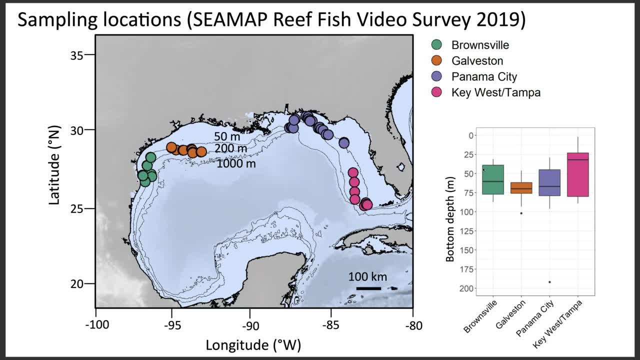 filtration method, like i i talked about earlier. that's shown in the lower right, um. so we've got, um, yeah, again, stations from key west, tampa area, panama city, and, you know, florida shelf, uh, galveston, as well as brownsville, so texas shelf, um, and so we see. 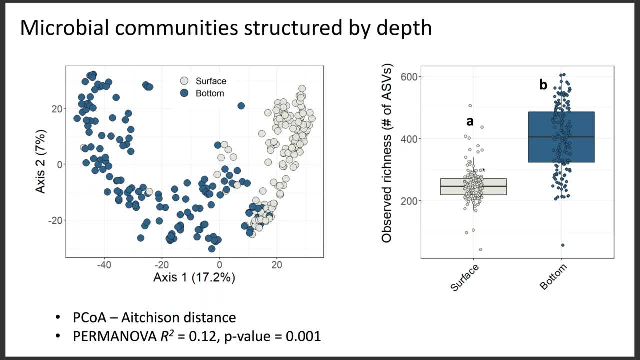 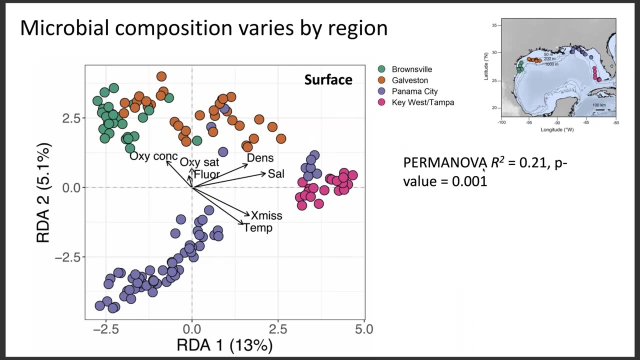 a really clear pattern between um surface and bottom, as, as we expect, um there's a lower diversity in the surface than in the bottom depths and they're clearly differentiated from each other, and we can- you can- determine that um oxygen and um and temperature are are driving a lot. 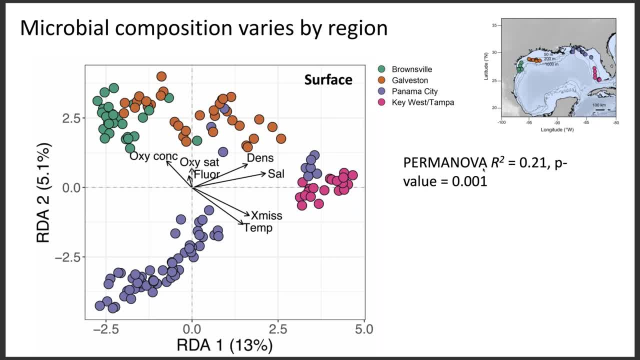 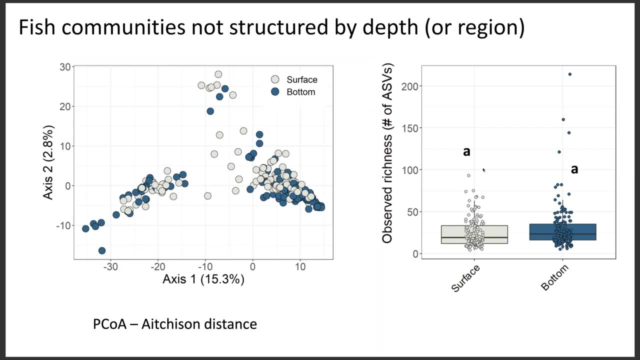 of the patterns and separation. so at the surface we see um pretty clear delineation between the different, uh, different regions, um, and so that's suggestive of some of regional separation: uh, uh, uh, um. so we're getting a lot more um, we're getting a lot more um information, um, uh uh. to go into a, 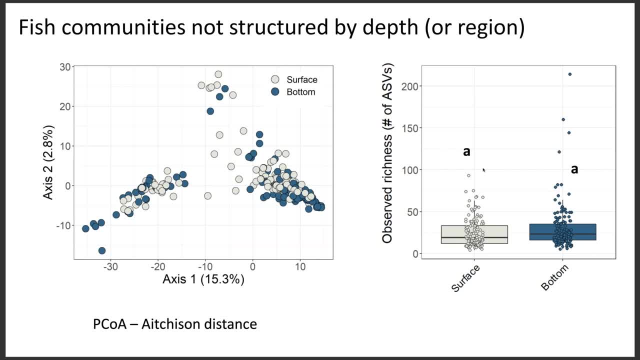 more132 um. um, at the上下半期. um, look at the center over here, uh, and we've got the average mpc. um, the mpc is about 90% of the round sand. but, um, what we're, uh, we're looking at, right. 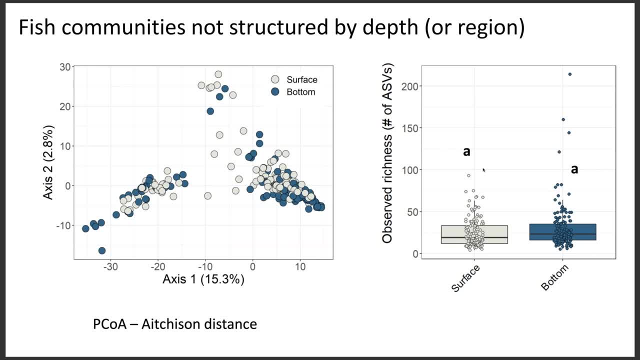 now is about 50% um of the round sand, which is only about two percent, but that's uh, that's uh, uh, a lot of the uh, um, uh, area of data, um that they're looking at, um, and then, uh, and we're still um, and i'm going to go on right now, um, and look at this slide. over here to the next slide, please. 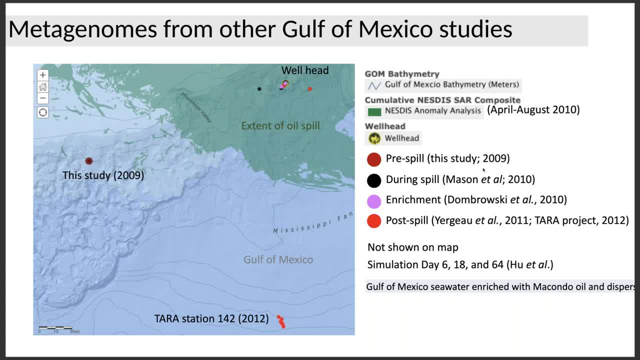 Finally, we have some data that we've been working on that dates back to the Deepwater Horizon spill, And so Jean Lim has been working on this with me, And so we have samples from around the wellhead area, and this were taken during or after. 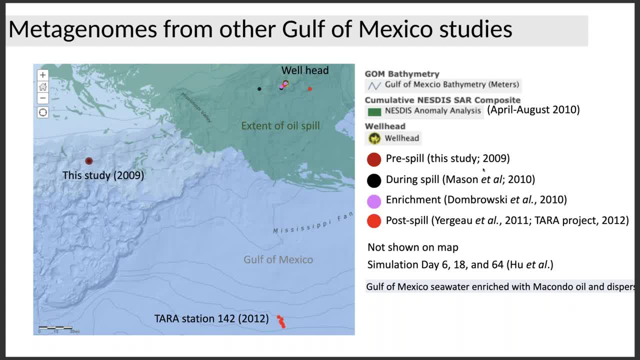 the spill, as well as samples that were enriched with oil, and to try to model the spill And the whole idea of this project. of course, the Deepwater Horizon spill was a horrible disaster, but we wanted to try to figure out what was the dominant microbes that were degrading. 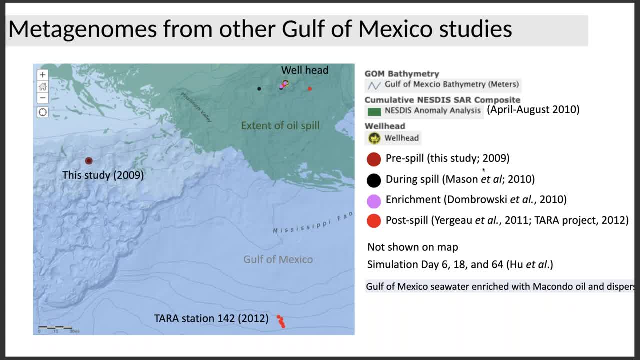 the oil And could we detect them before? And essentially we could not find the exact microbes before the spill that are now thought to be the ones that were degrading the oil. after the spill There's just very little abundance And that's interesting because it suggests that, I mean, we know they had to be there. 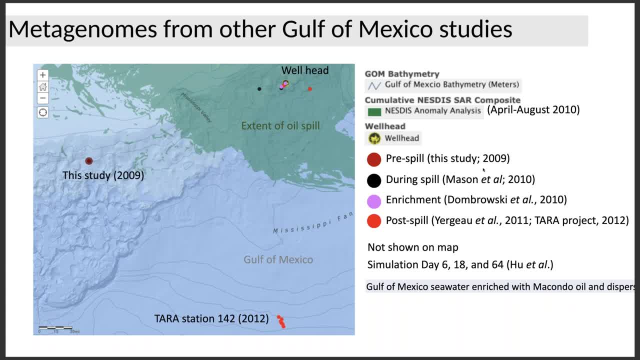 They started growing when the oil showed up, but they were at such low abundance That they couldn't be detected before the spill And this kind of gets at this idea. in microbial ecology it's called the Bosk-Becking hypothesis. 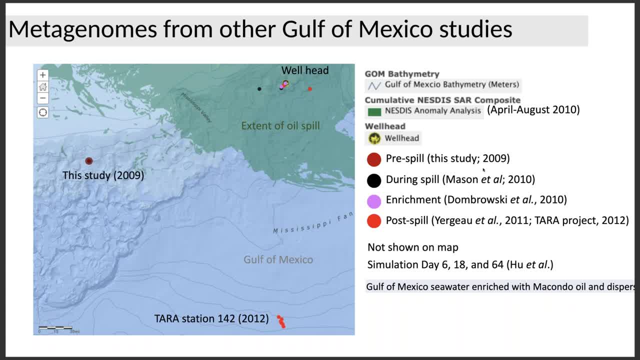 that everything is everywhere, but the environment selects, And so those microbes were present, but they couldn't be detected because they were in such low abundance. They hadn't been selected by the environment. So, in any case, what I'll just show here is that 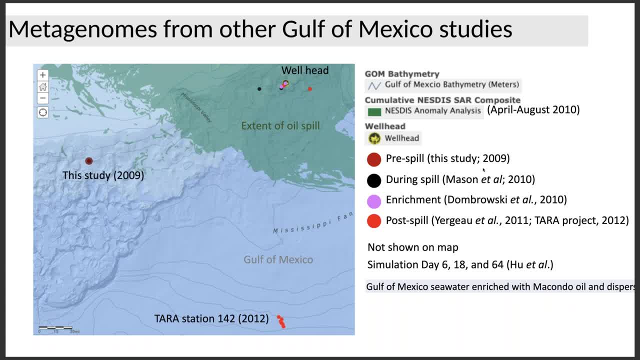 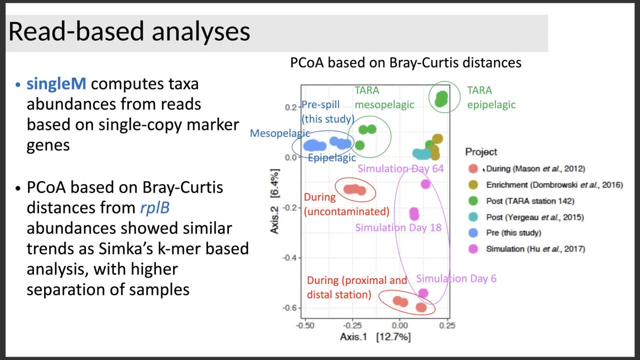 Okay, So this is a gene that's been used in some different tools to study these metagenomes and seeing some interesting patterns. So this one is based on a tool called SingleM that computes taxonomic abundances from reads based on single copy marker genes. 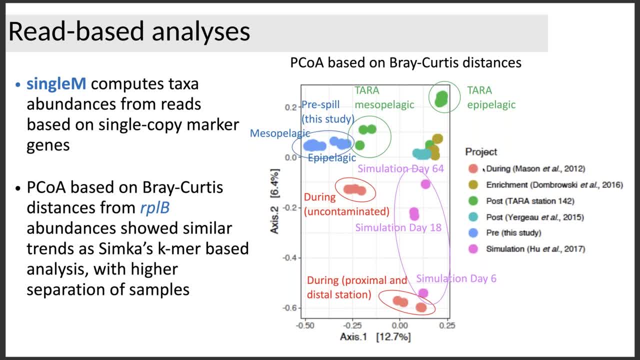 This is based on a gene called RPLB, And then we can do an ordination on these And so we see some interesting patterns, But important, Importantly, the pre-spill samples. they look like any other surface or epipelagic or 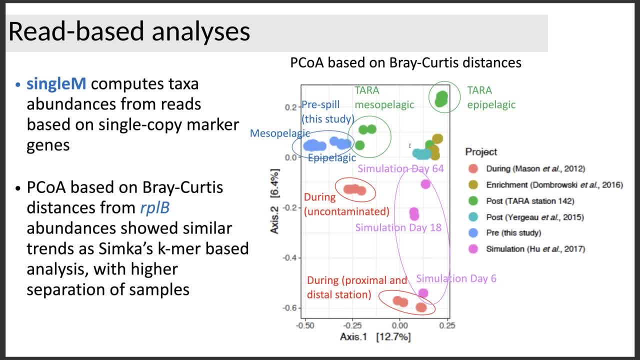 mesopelagic metagenome from the Gulf of Mexico. These TARA ones in green are also from the Gulf of Mexico from a little bit later after the spill, but still normal looking metagenomes, And so from both this Analysis and more in-depth analysis using read mapping, there was no pattern of sort. 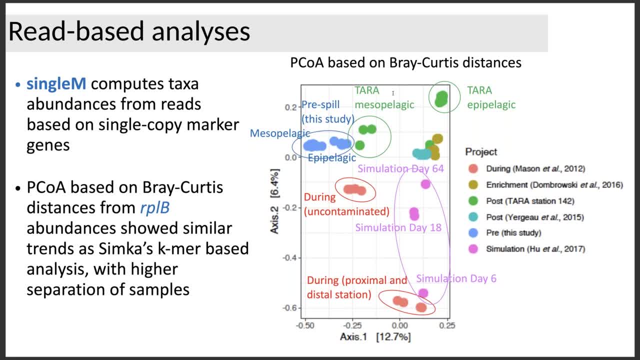 of being able to predict those functions of degrading oil before the spill happened. We know they had to be there because they started growing and were able to degrade the oil relatively well once the oil showed up. but in a normal seawater environment in the 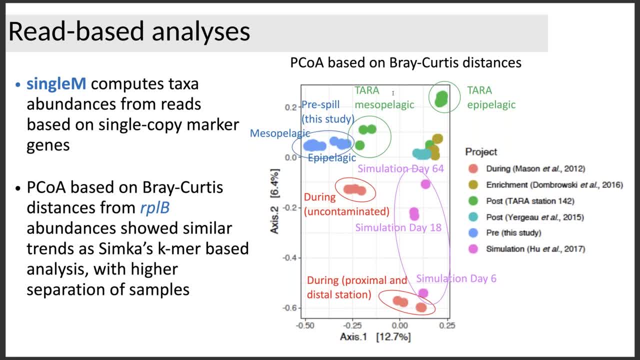 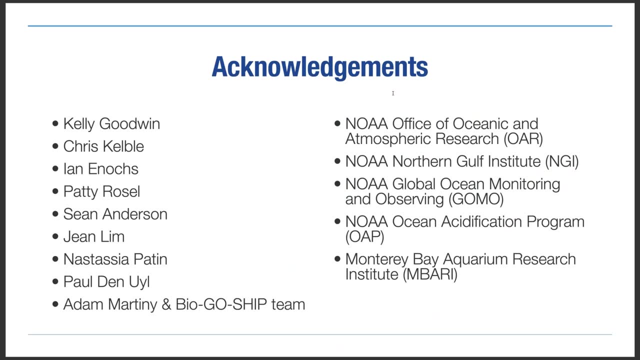 Gulf of Mexico. I don't think we have any more data on that unless you're closer to hydrocarbon seeps and that sort of thing. They're pretty low abundance And so that's all I have for today. Wanted to thank a lot of different folks at NOAA and collaborators for their help and 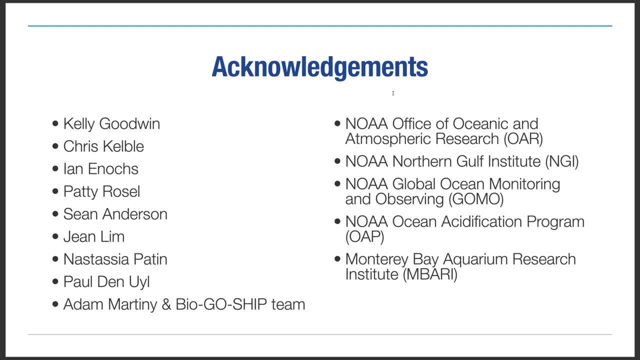 contributing to this, to the science that I shared today, and especially want to thank a number of different NOAA. Thank you line offices and programs that have contributed to this work, in particular OER, NGI, and I should say OER, N-O-E-R, as well as NGI, GOMO Ocean Acidification Program, and then 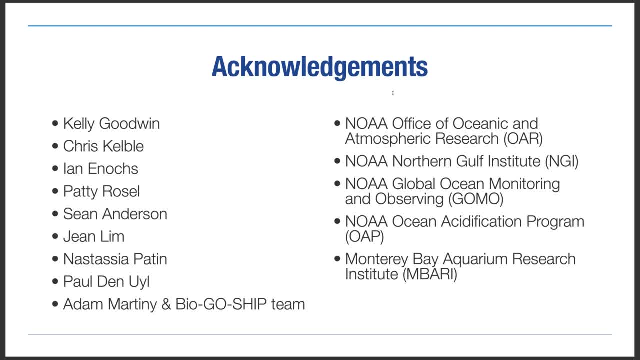 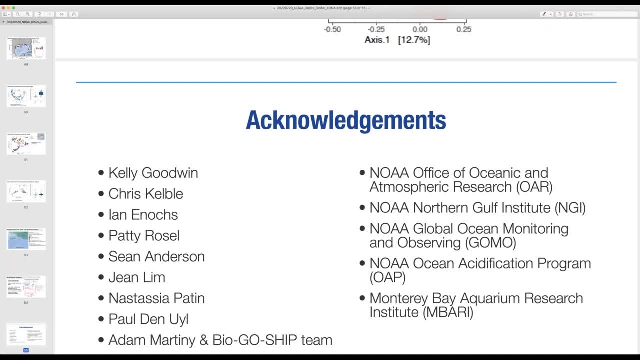 our collaborators at MBARI. So, yeah, I'll leave my slides up, I guess, in case there's questions, but I'm happy to answer questions in the chat or out loud. Excellent, Thank you so much, Luke. That was a fantastic presentation. 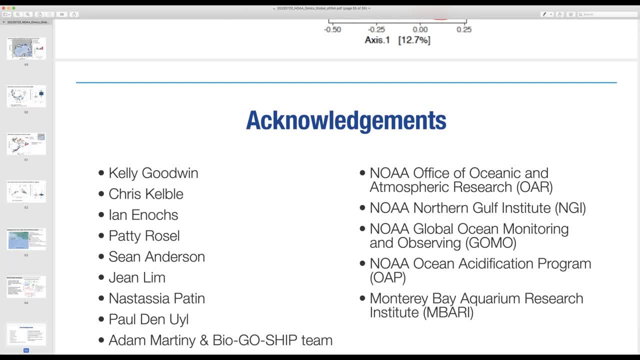 Yeah, folks feel free to type questions into the questions for staff box and I'll read them out loud for Luke to answer. We do have one question that came in earlier, Luke. This one's from Carol. She says: Luke, great talk. 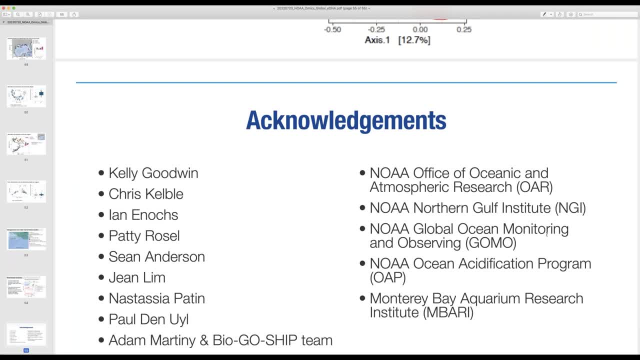 Please tell again what your differentiation is between metagenomics and multi-gene, multi-sample meta-barcoding. Yeah so yeah, with meta-barcoding you can do multiple genes or multiple targets. So imagine you have a seawater sample. 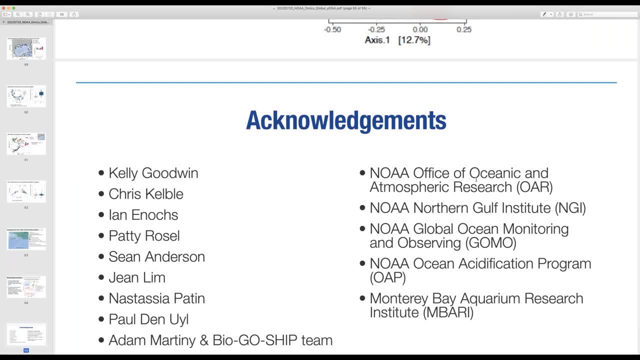 And you've extracted all the DNA from it, and so it should be full of bacteria and plankton and maybe some traces of fish and whales and viruses, and anything that might have ever been in that water could be in that DNA sample. So with meta-barcoding, you can choose which gene you want to target. 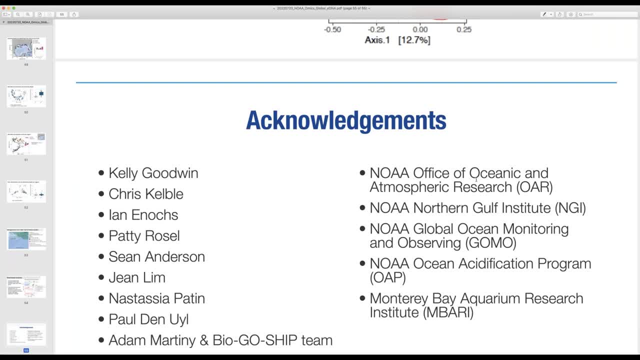 Say: you want to go after bacteria, So you use the 16S RNA, the small subunit, And then you can go after bacteria. So you use the 16S RNA, the small subunit, And then you can go after bacteria. 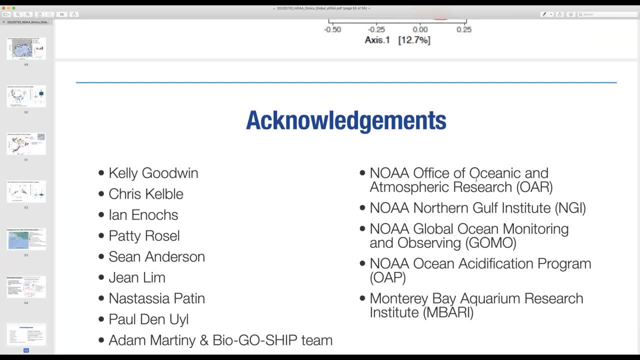 And then you can go after bacteria, Or you want to go after fish, so you choose the 12S RNA, which is also the small subunit but of mitochondria of fish, et cetera. So each one of those will give you a different picture, because those primers will ideally 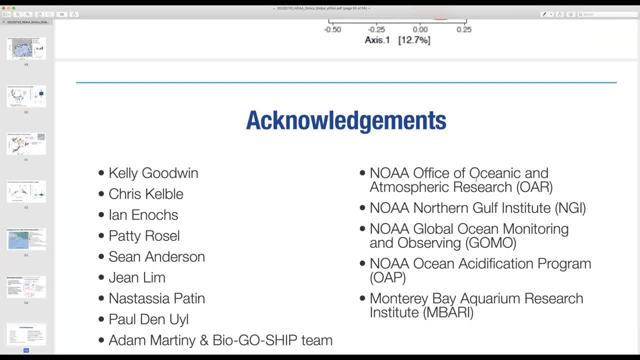 only amplify that taxonomic group. So you can analyze those data sets together So you can look at co-occurrence patterns. There's a little bit of apples and oranges, but they are each a profile of a given taxonomic group or large taxonomic group. 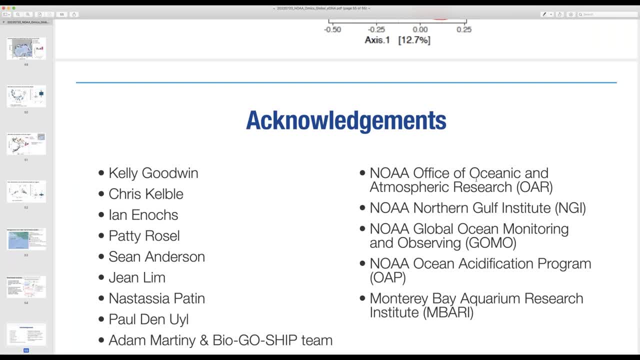 And then with metagenomics you've kind of got everything there, So you might miss out on some of the rarer stuff, like fish for example. Those might not show up just because you have so much more bacteria that are in that. 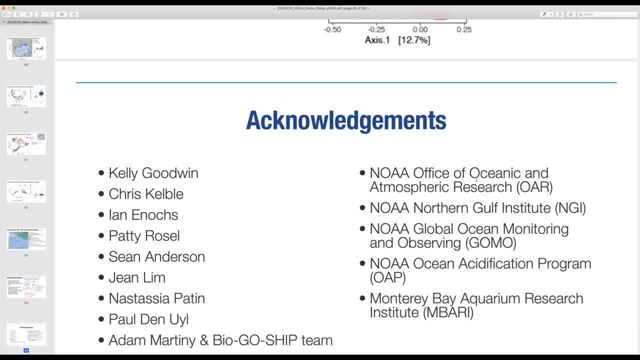 group, And then you can go back to the material DNA, But then OK, maybe you do have everything there at some level, and then you're still going to need to do some sort of profiling. So that will also be dependent on the database. 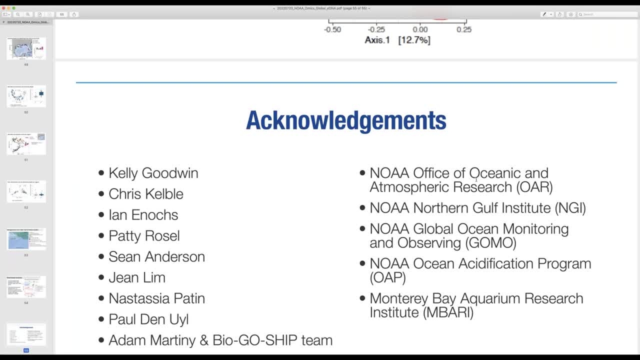 And if you do assembly you're probably more likely to assemble those bacteria or things that are more abundant. So I don't know if I answered the question, but basically there's… You can do more with metagenomics, but you're going to potentially miss out on the rarer stuff. 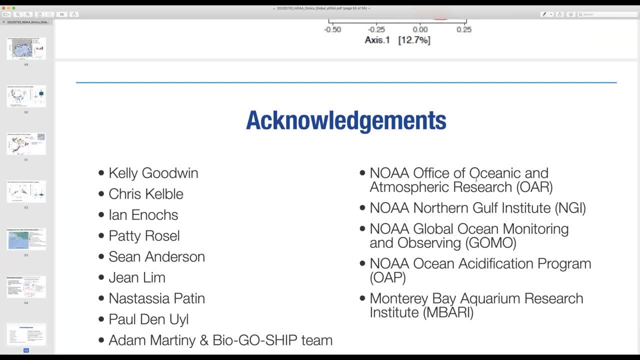 And you're going to need to do a lot more. The algorithms are more. there's many more algorithms and they're more complicated, But ultimately it's going to be more rewarding because you can get functional information as well as taxonomic information, and that's pretty useful. 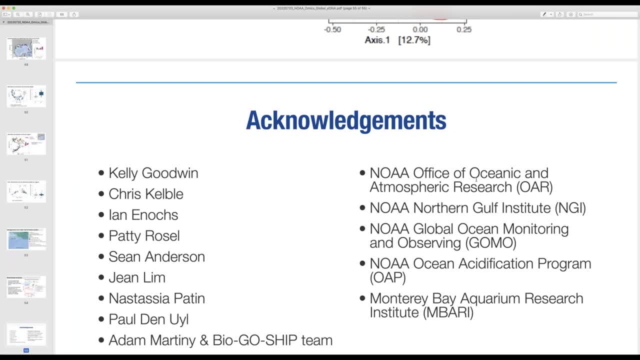 Excellent. Thanks so much, Luke. We had another question that came in. This one's from Victoria. She says: Hello Luke, Great talk. Thank you for your time. How can we get in contact regarding your work and joining your team? 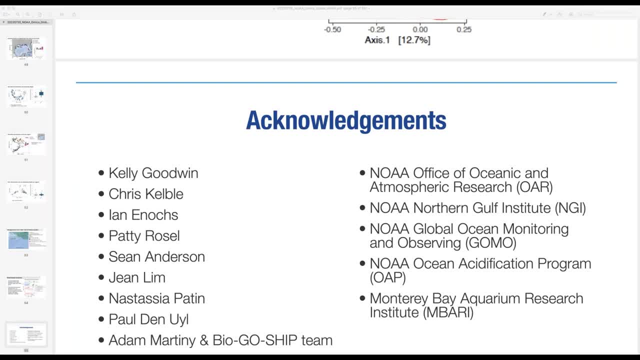 Oh, great, Yeah, just send me an email. I can put it in the chat. Would I send it? Would I do this to organizers and panelists? or Catherine, Yep, yep, Yep, Send it out to all attendees. 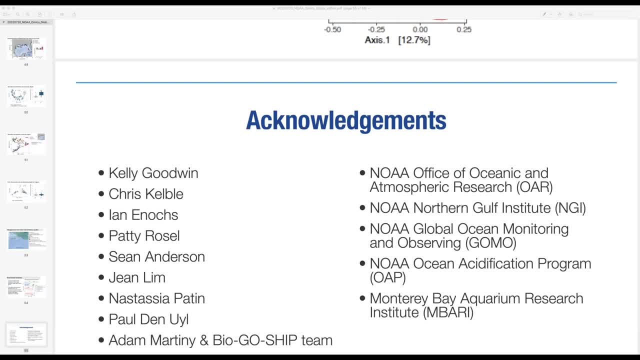 OK, I'm not seeing that as an option. I see organizers and panelists. Oh, I can. I can put your email here in the chat, Luke, So I got it. Do we have other questions from folks in the audience? OK, I'm not seeing any come in. 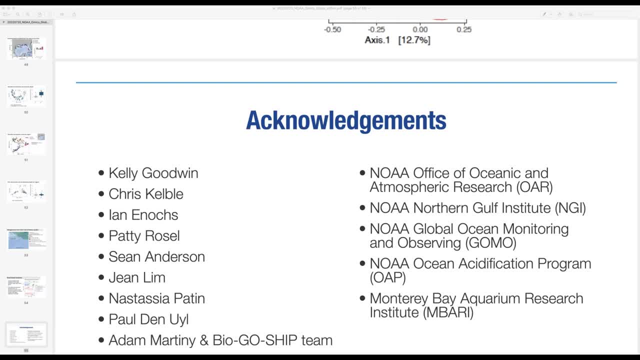 But here's Luke's email. Oh OK, I see We both put it in the same time. OK, good, Oh great, Yeah, So, as I mentioned at the beginning, we're hiring, So we've got one postdoc that's going to be focused on the BioGo ship and MBON work. 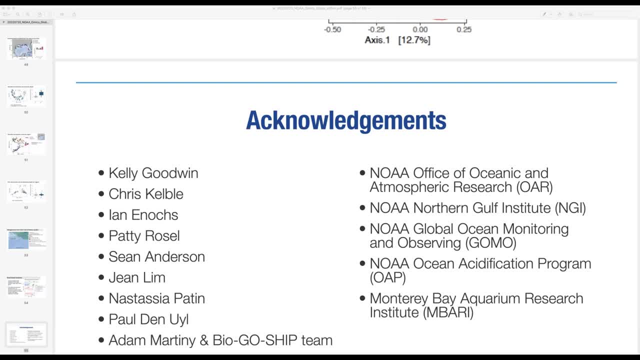 And then we have another project on sediment traps to study the biological carbon pump, And we haven't- And there's some links there to ocean acidification, foraminifera, Some different things, Yeah, Yeah, So we have some really cool angles there. 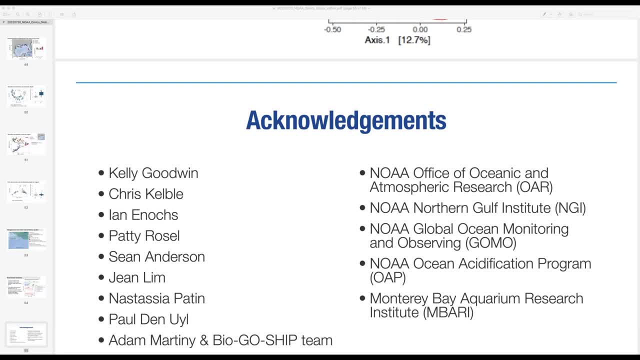 That's a joint project with Emily Osborne at AOML, And so we have a postdoc to work on that project as well. In addition, we're going to be hiring a project manager to use more of a bioinformatics PhD level, But sort of floating between different projects and running our HPC effort using some of the like the supercomputer we have at Mississippi State Orion. 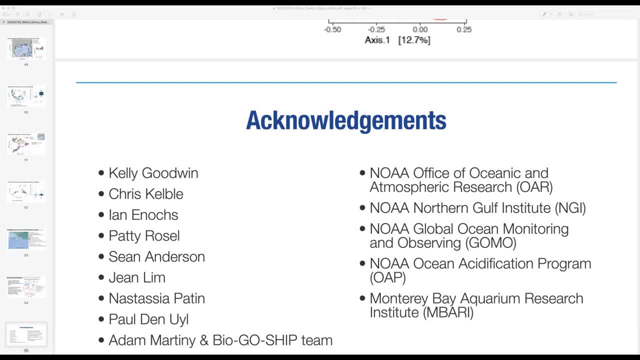 So that's going to be a third position that's more of a project manager, but heavily bioinformatics. And yeah, we're also looking to hire a technician who's going to be doing some of the SASE work and general molecular biology stuff in the lab as well. 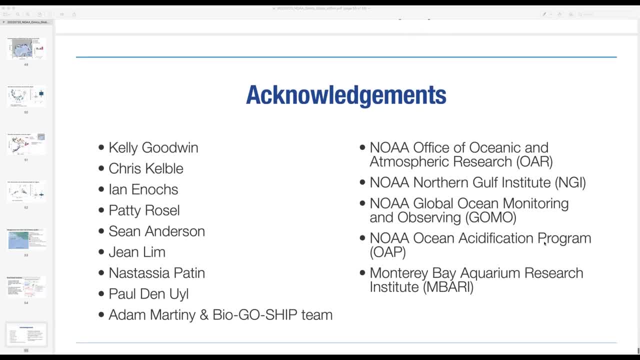 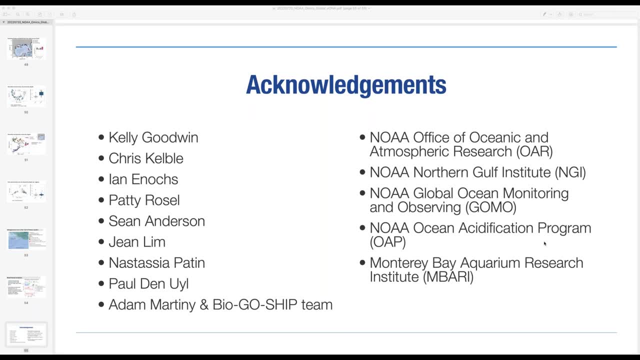 Awesome Thanks, Luke. I actually just put a link to AOML's career page in the chat. If folks want to flag that, I think a lot of the positions supporting or working at AOML will pop up on this page. 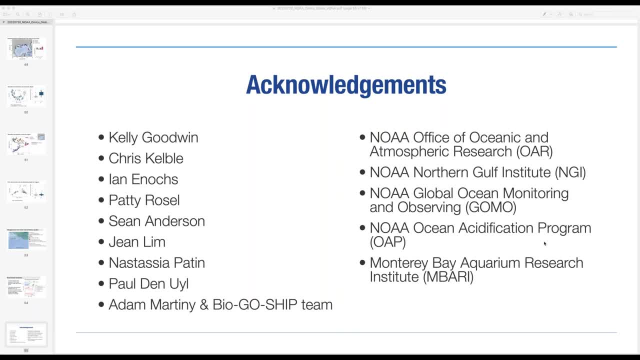 And I think folks can also check USA Jobs and the University of Miami career websites to look at these upcoming positions And also Mississippi State job board, because those first three positions will be through Mississippi State But they'd be based in Miami. So, just like me, I'm a Mississippi State employee but I'm based in Miami. 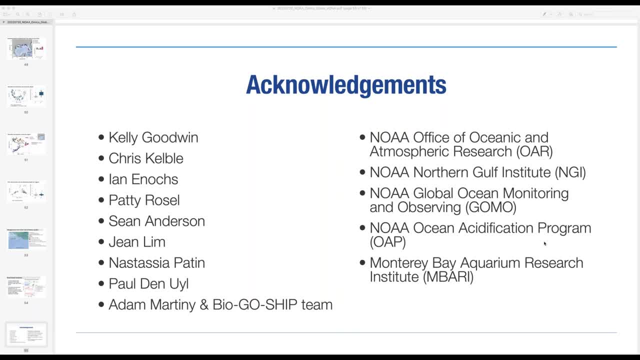 Awesome. Okay, I don't see any other questions here, But if folks do have lingering questions, please reach directly out to Luke. His email is here in the chat, And so Luke just want to say thank you so much again for presenting today for the seminar series. 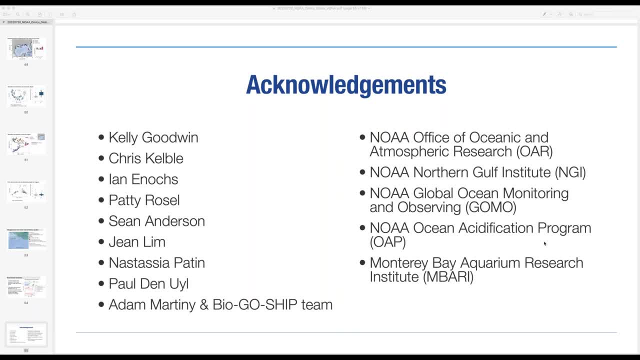 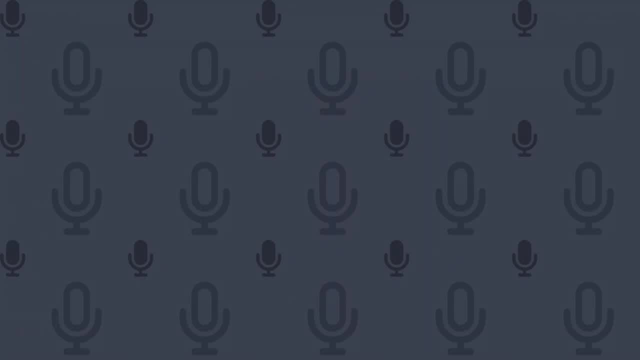 And I want to thank everybody for joining us today. Our next seminar is on August 19th at 1 pm Eastern Time. So this is a different from our normal seminar time, which we have. it normally is at 12 pm. 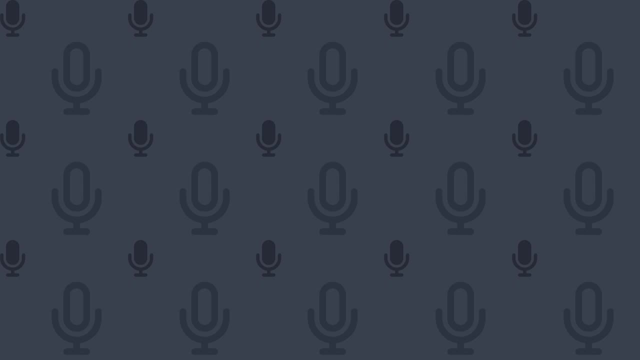 So it's at 1 pm, August 19th. Please visit the omics website to get information on how to register for that talk. This one is going to be by Dr Ingrid Spies from Noah's Alaska Fishery Science Center. 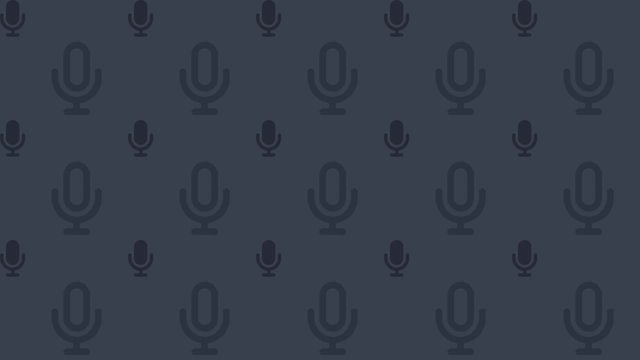 So thank you all again for joining today. Have a great rest of your day. Thank you, Catherine, Thanks everyone.